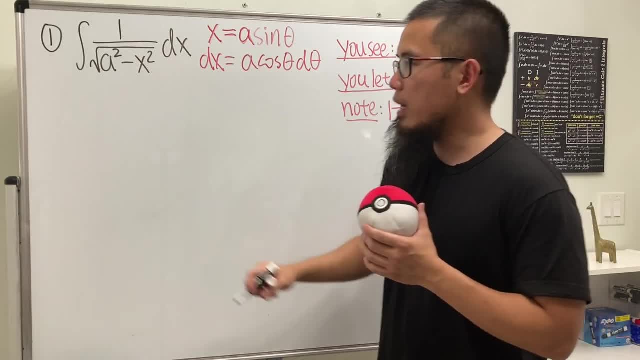 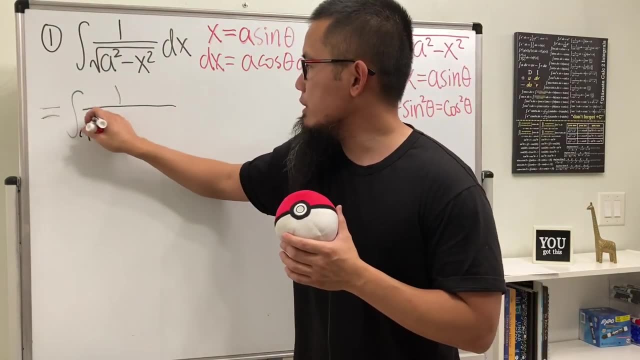 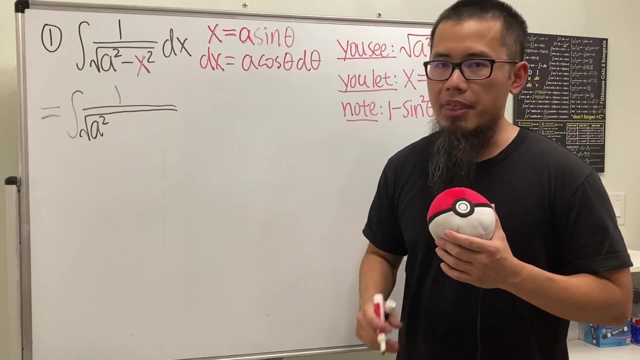 we can just now take this integral to the theta world and we're looking at the integral of 1 over square root and here we have the a square. but this x right here is what we say to be a times sine theta. So we're just going to write that down a times sine theta and then we have to square. 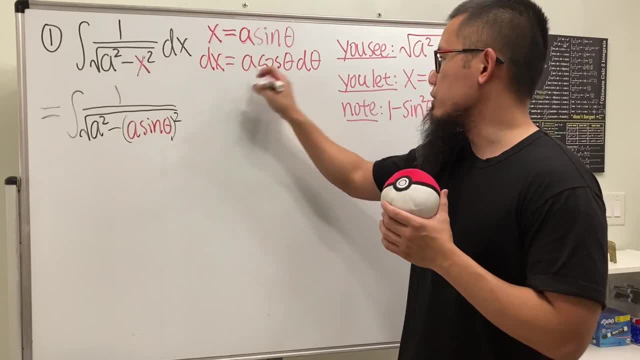 that. and we see we have the dx right here, which is all that. So just be sure that you multiply this right here. and then we have the dx right here, which is all that. So just be sure that you multiply this right here. 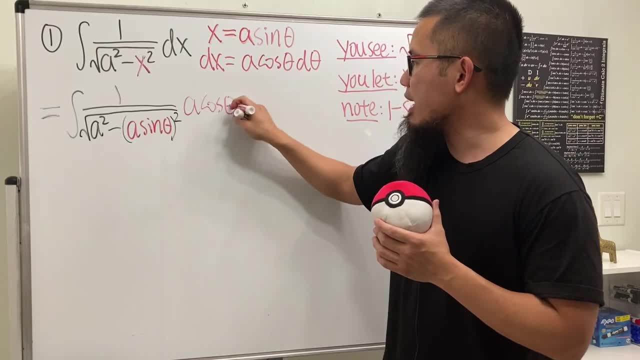 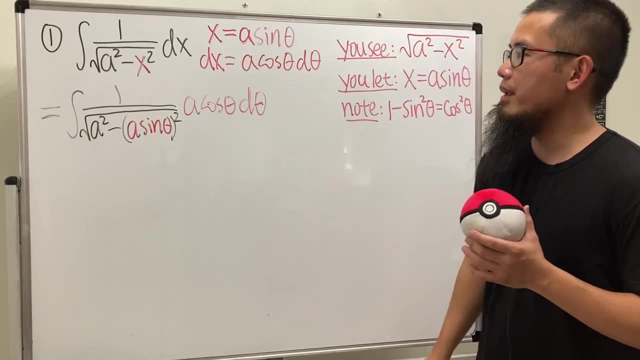 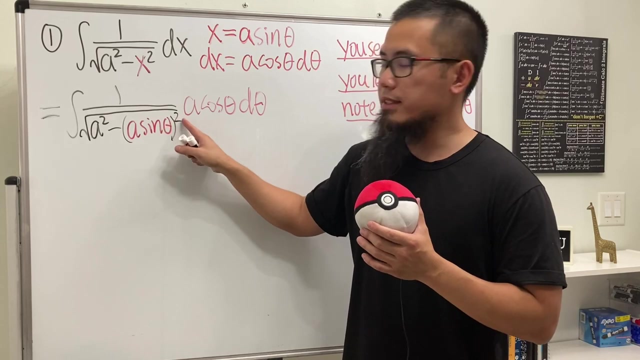 right here as well. a times cosine theta, d theta. Do not miss the d theta. that's extremely important. I will point out why later. So this is what we have now and now we can simplify this a little bit. Here we have a square and we also have a square right here, so we can factor that. 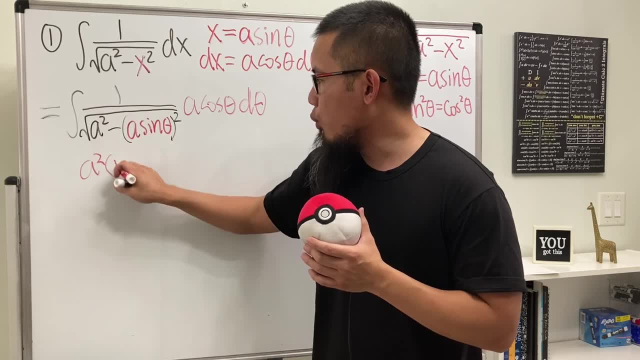 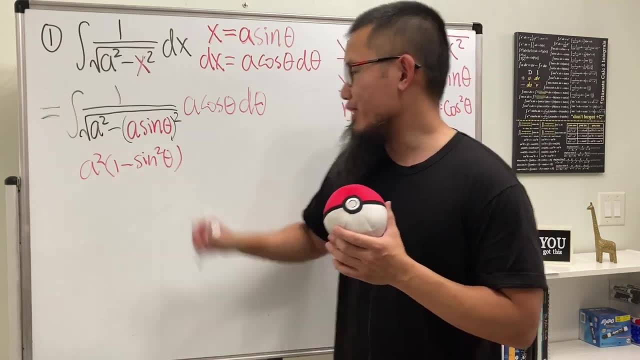 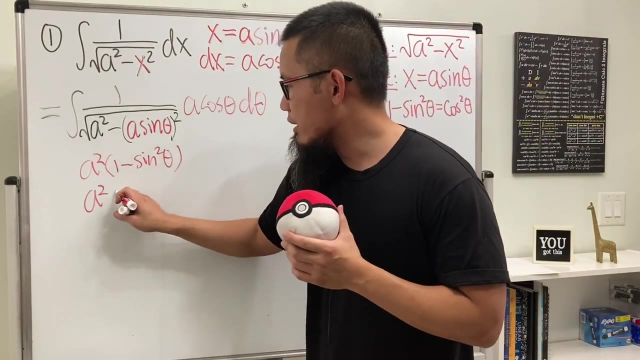 out a square and then we will just have 1 minus. here we have sine square theta. Well, this right here is what I told you. we'll be expecting to use this identity, so we can replace that with cosine square theta. So this is just a square times cosine square theta, and you have to keep in mind. 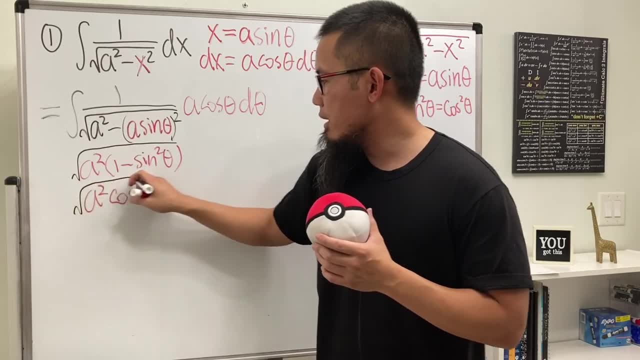 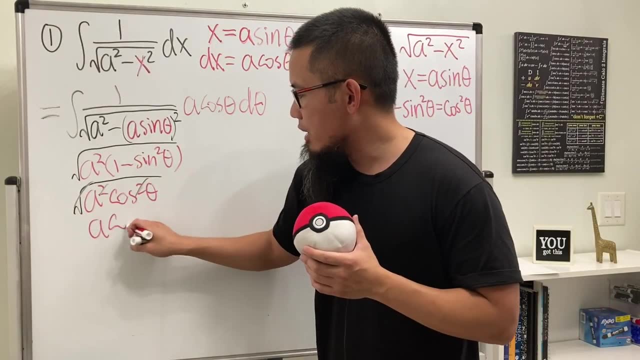 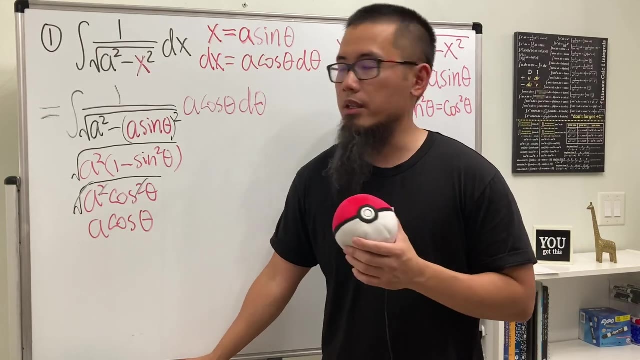 this right here, is still inside the square root, right here, right, And the beauty of this is that this can still out. So, all together, we just get a times cosine theta and you don't have to worry about the absolute value for this integral, because we're just trying to find an antiderivative for 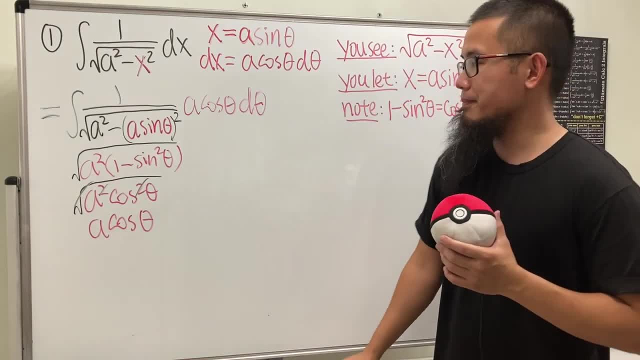 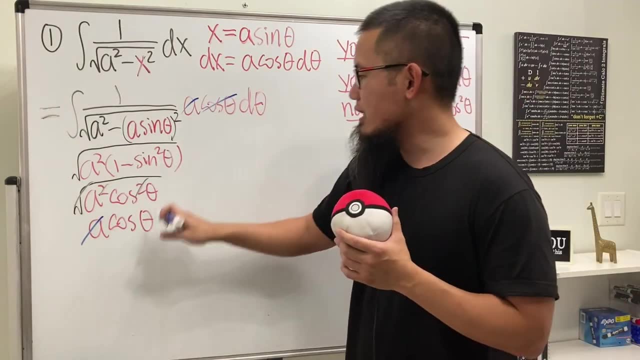 this All right, and now here's the best part: a here, and then we have a on the bottom, so we can cancel them out. Likewise, cosine, cosine, cancel each other out. So we actually just have to integrate. 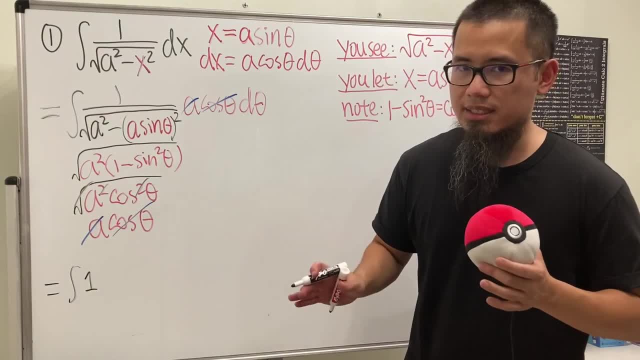 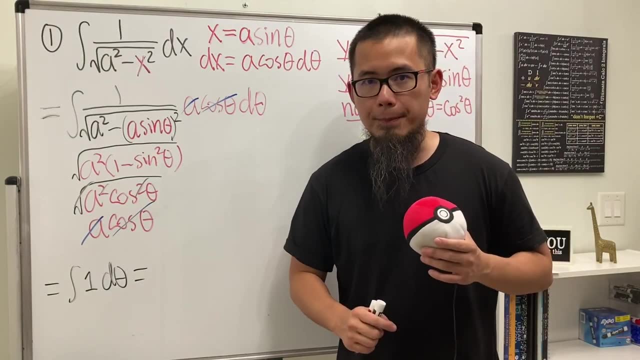 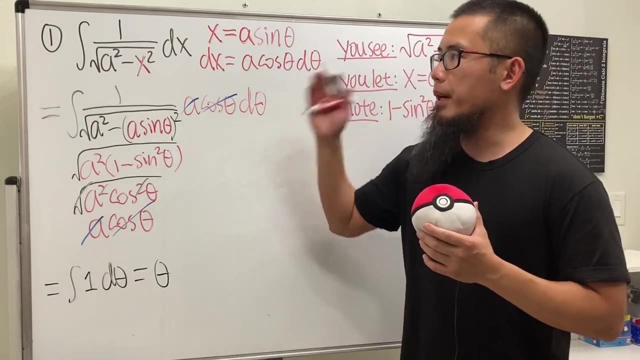 1, but the answer for this is not just x, because we are in the theta world, So really be sure to write down dy every single time, Integrating 1 in the theta world. we actually get in the theta world. we actually get 1 in the theta world, but we still have to go back to the x world. 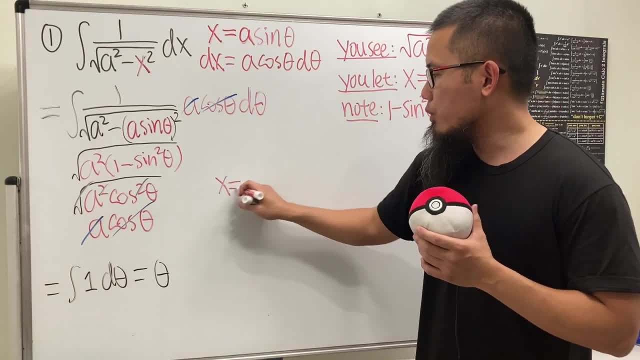 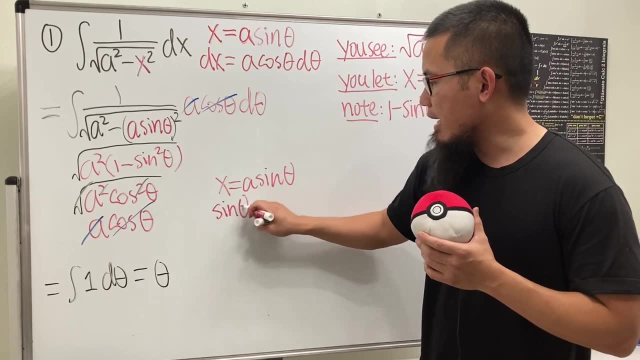 and to do so we just have to look back here. We know x is equal to a times sine theta. This means we can divide a on both sides. so sine theta is equal to x over a, and right here we can just say: 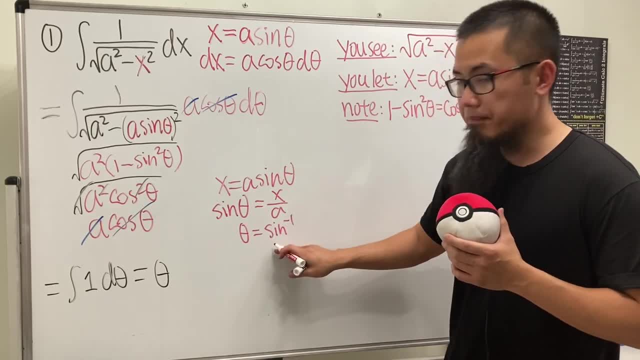 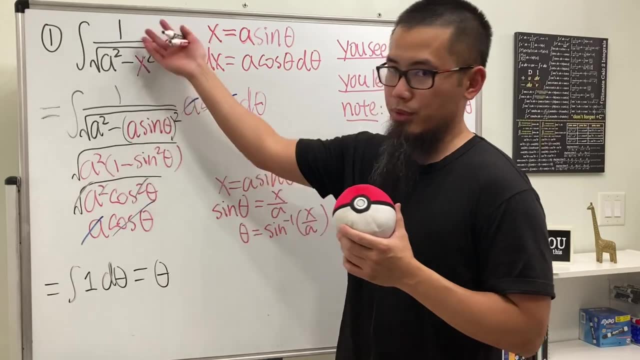 theta is equal to the inverse sine of x over a. So, ladies and gentlemen, this right here is just the theta, which is pretty much the answer for that. So I'm just going to write that down right here for you guys. Final answer. 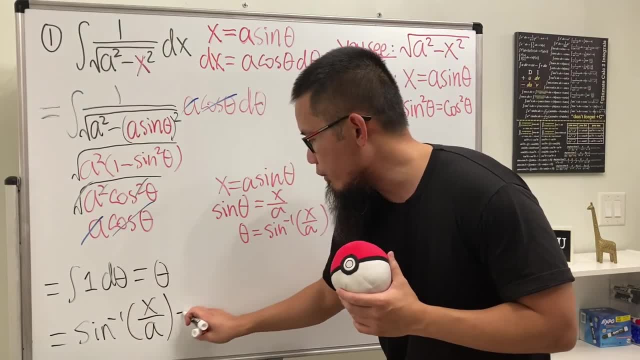 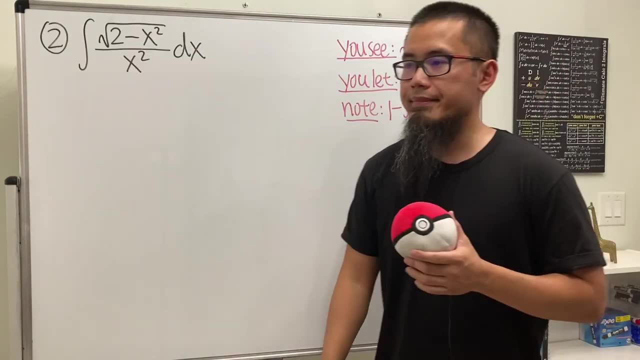 inverse sine of x over a, and then we are all done. So I'll just put down a plus e right here and box the answer just like that. For number 2, we have the integral of square root of 2 minus x. 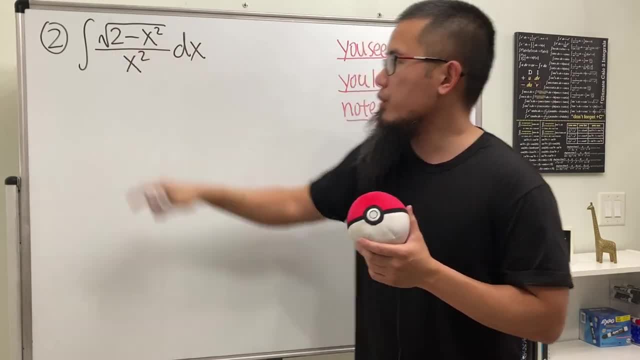 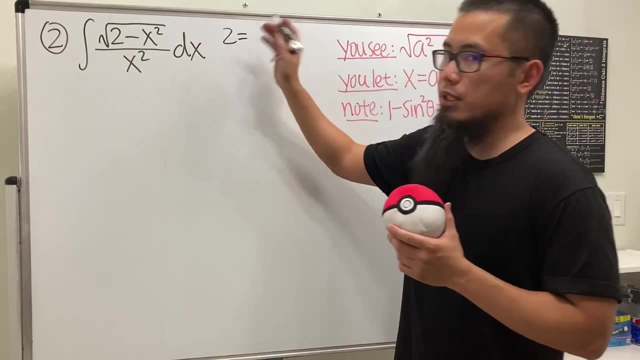 squared over x squared. Here we have this number 2, and we really have to look at that number as a number to the second power. So the truth is, for the 2, we'll just purposely look at this as square root of 2.. 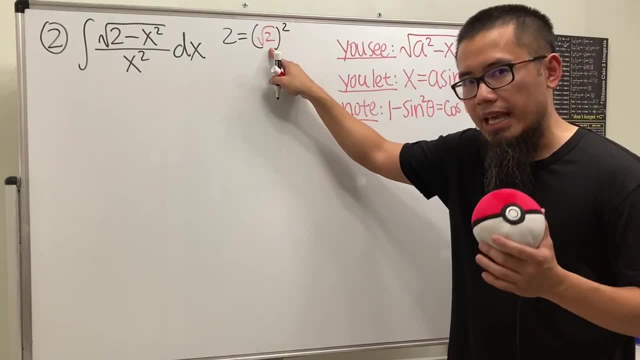 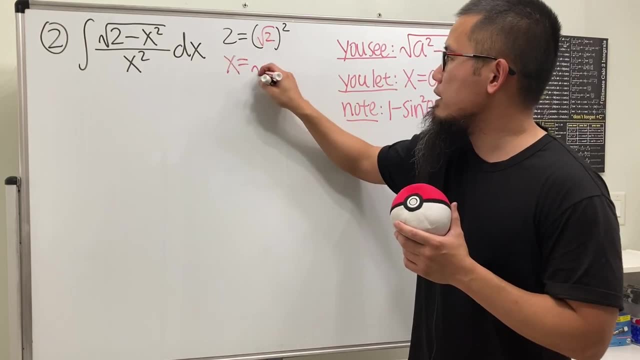 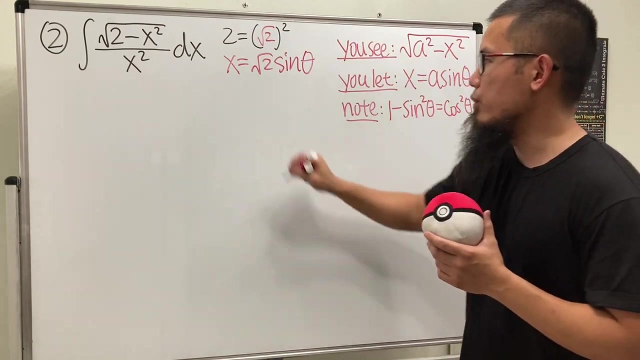 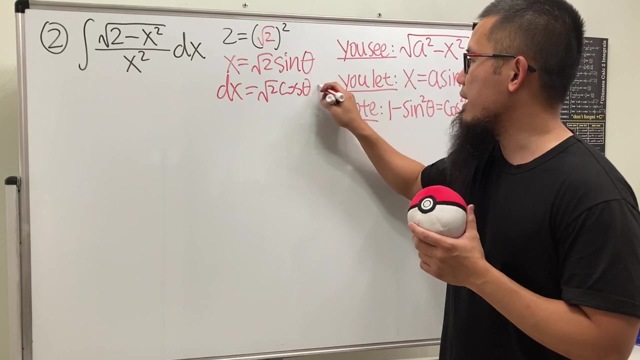 and then square. so this tells us the a is square root of 2. so here you see, we have that. so we can just go ahead and say x equal square root of 2 times sine theta, and then just continue the usual business: differentiate that and then we just get square root of 2 times cosine theta. 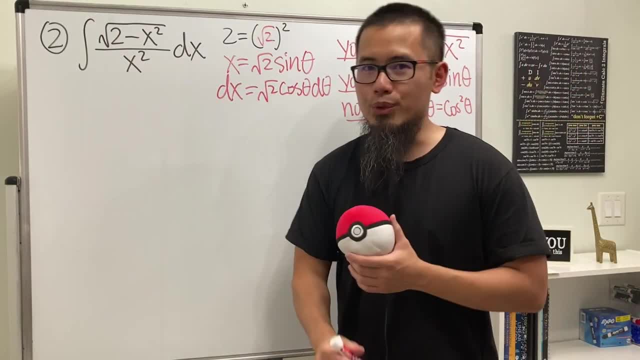 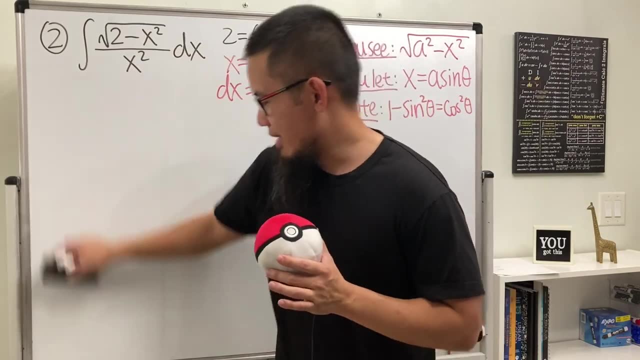 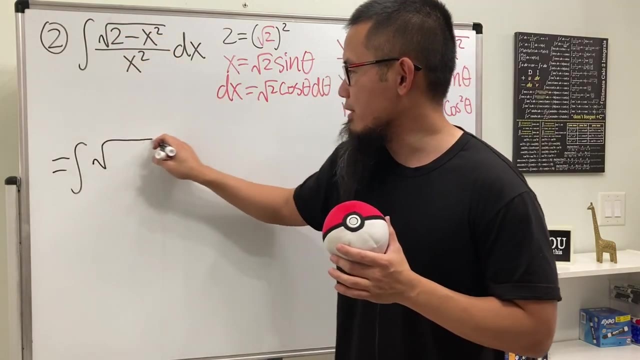 d theta and, of course, take this integral to the theta world. so we are looking at this as the square. i'm going to actually leave some space right here. i almost forgot about that. leave some space because we have the square root on the top and i'm going to simplify the square root expression. 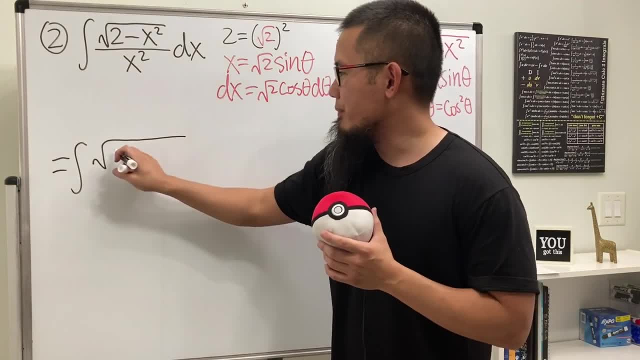 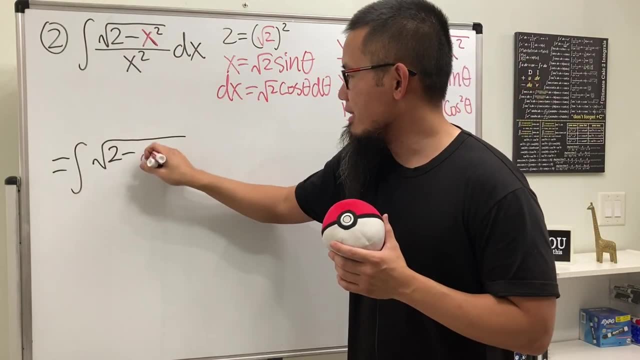 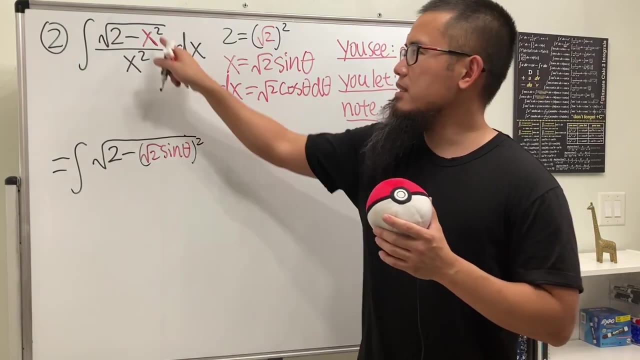 so let me leave some space right here. anyway, here we have 2 minus. take a look right here. this x is what we said. it would be square root of 2 times sine theta, and then we have to square that and you can see if this is to the third power you would. 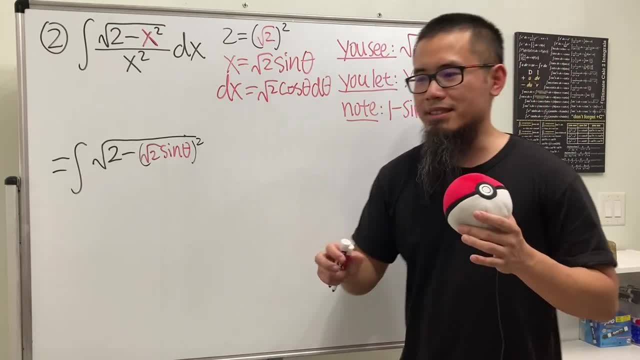 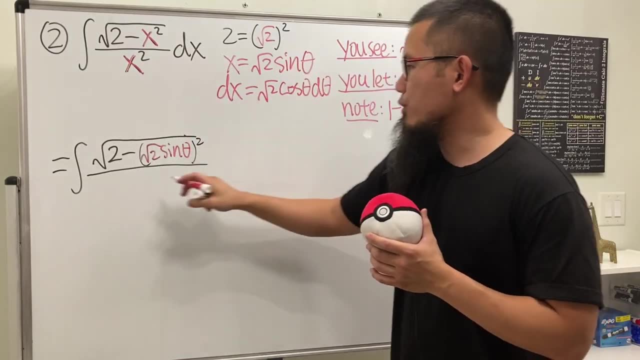 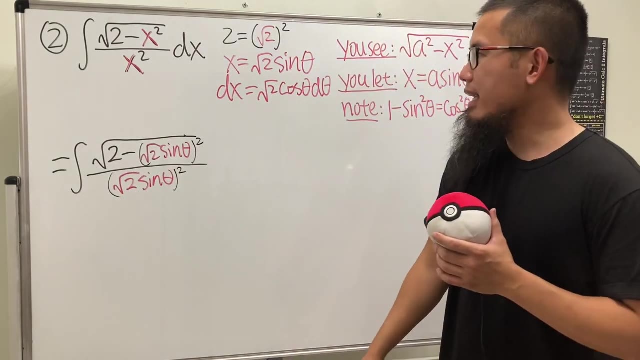 know that it's not going to work out. so, just just like it's so nice, the second power, right, all right. and then on the bottom, here we have the x square, and the x is going to be that square root of 2 times sine theta. and then we square it- and don't forget that dx is all that. so we multiply. 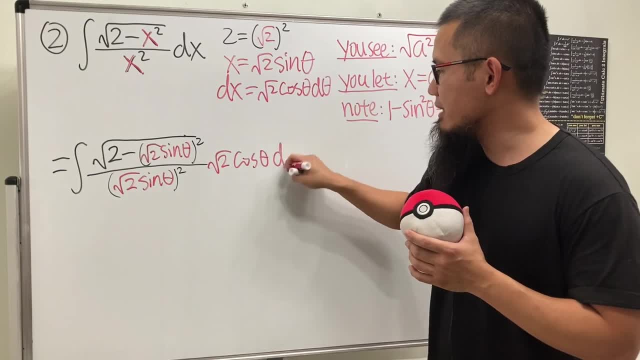 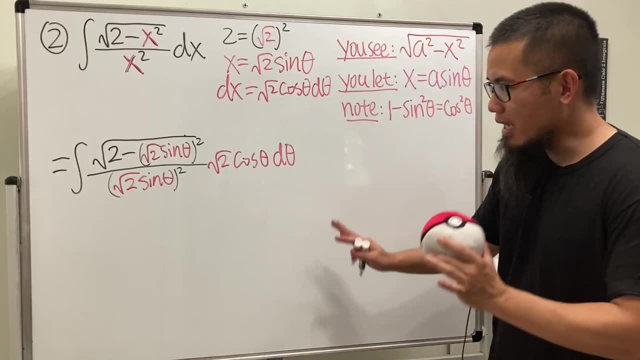 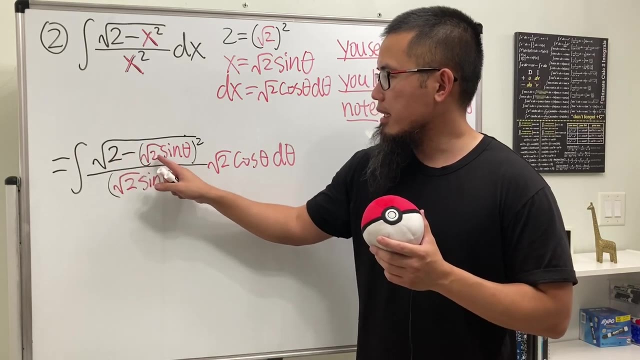 by square root of 2 times cosine, theta, d theta. wow, i know it's quite a lot, but uh, don't worry, just kind of, you know, relax, and then we can finish this. okay to do so. here we see 2 minus, and this is just a 2 right because square. 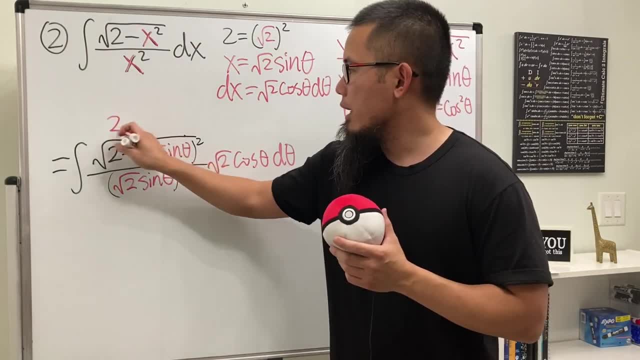 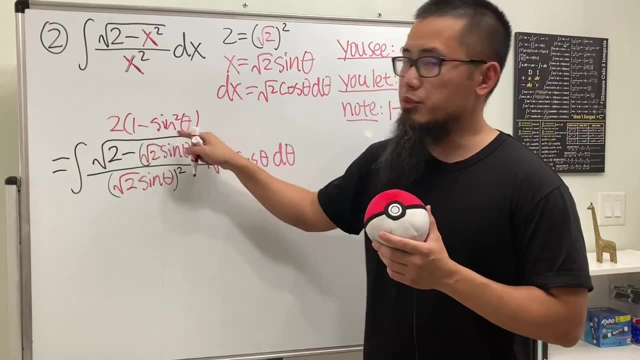 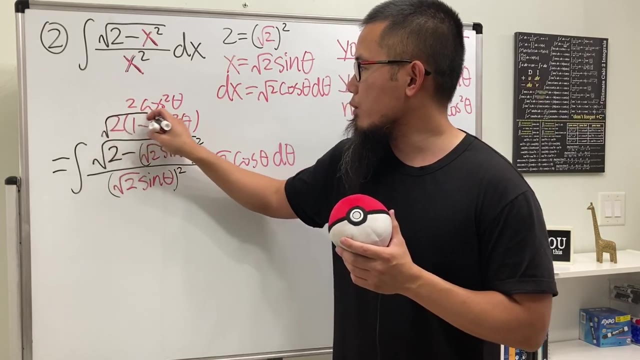 root of 2 square is just a 2, so we can factor that out and then we get 1 minus. this is sine square theta and this right here is again cosine square theta. and then we have the 2 in front like this, and remember, this is the square root, like: 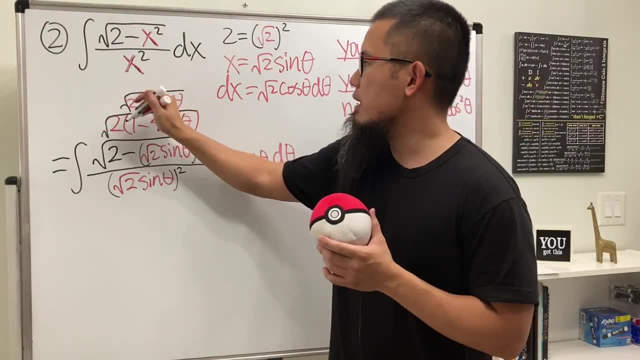 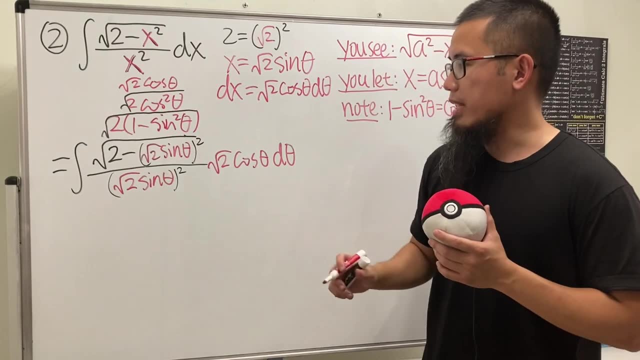 this and the square root of 2 will just db as how he is. so we have square root of 2 and this right here they cancel. so just have cosine theta. so that's for that. and if you look at the bottom, here we have square root of 2 square. 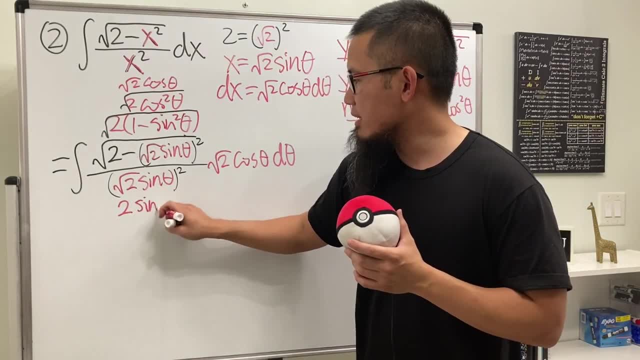 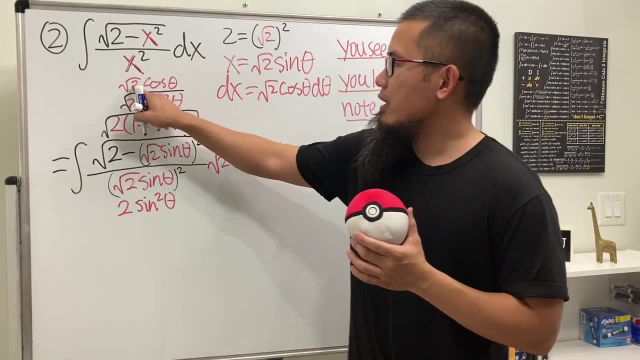 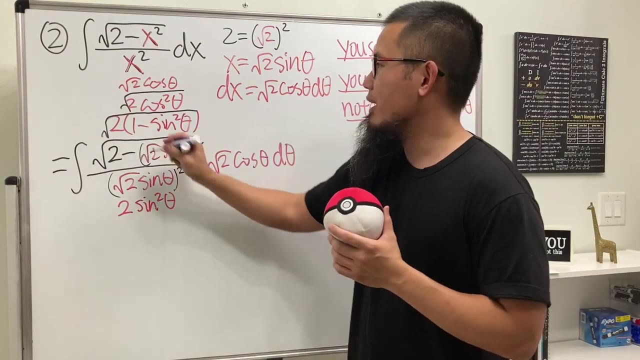 which is just a 2, and then this right here is sine square theta, alright. so this is- we have check this out- square root of 2 times square root of 2 is a 2. that's on the top, but here we have another 2, so they actually all cancel each other out, all right. and then, if you look at, 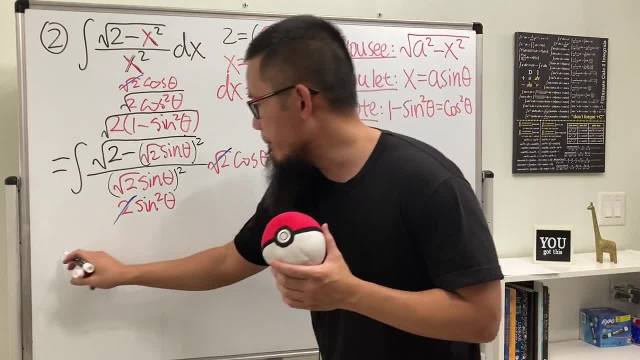 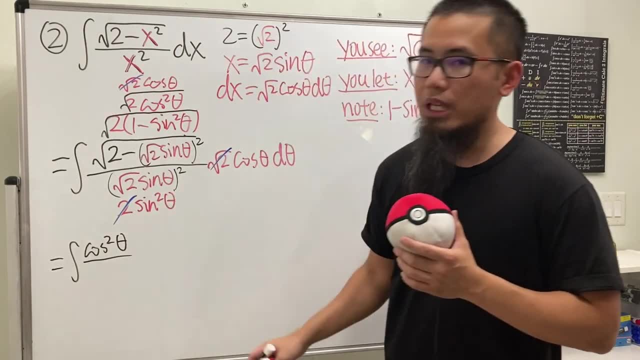 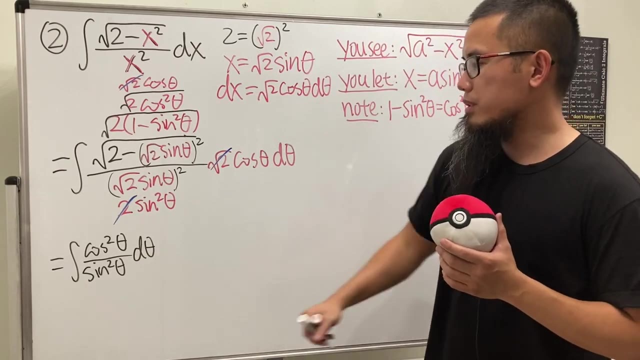 this time stat is cosine squared theta. i'm going to write that down to make it super clear. on the top we have cosine squared theta. on the bottom we have sine squared theta and then d theta and of course you can recognize this as cotangent square theta. and 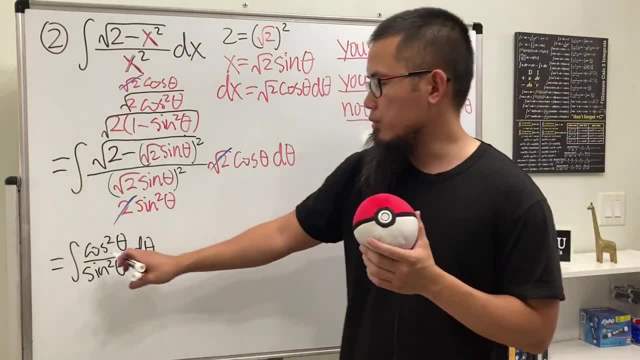 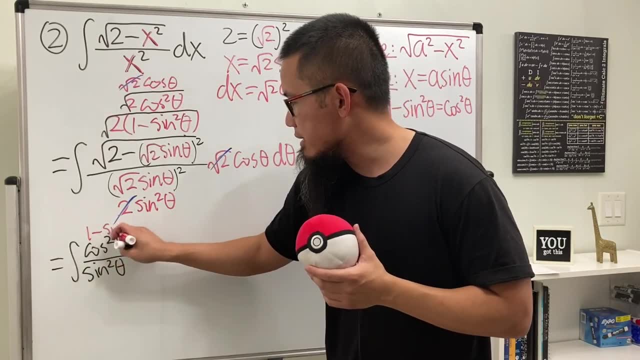 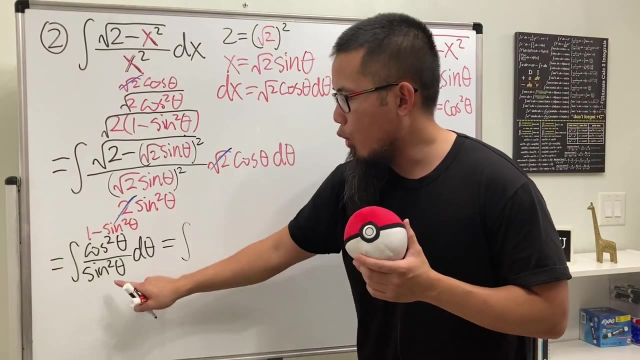 they can use the identity to break it apart. but i would just like to just prove that little identity for you guys. real quick: cosine squared theta is the same as 1 minus sine squared theta. so this is what we get first. we do one over that and that will give us. 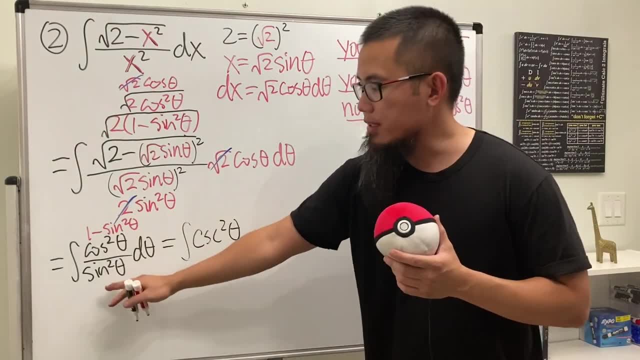 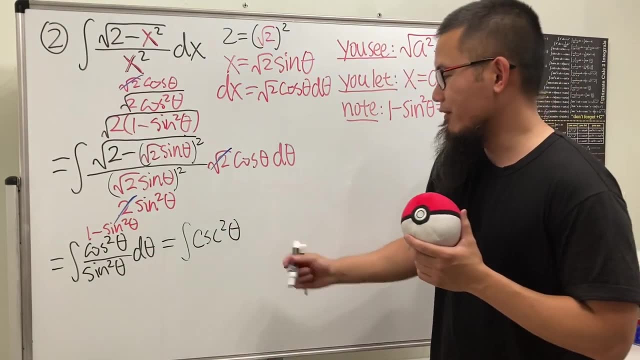 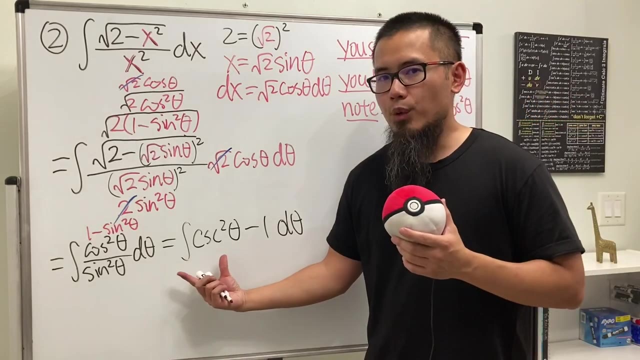 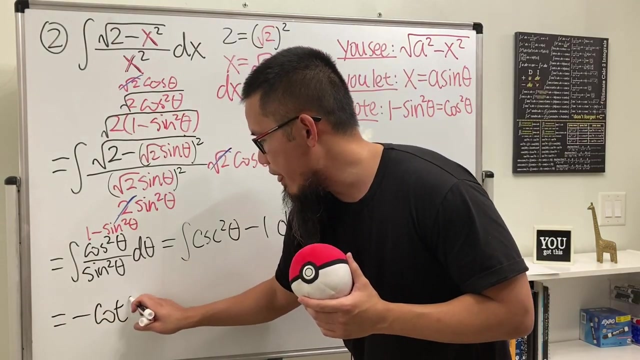 cos square theta, one over sine cosecant, but this is the square, so we have the square next this over. that is just one right. so very nice. so we have that minus one again. we are in the theta world like this. now, what's the integral of cosecant square theta? well, the answer for that is negative cotangent theta. 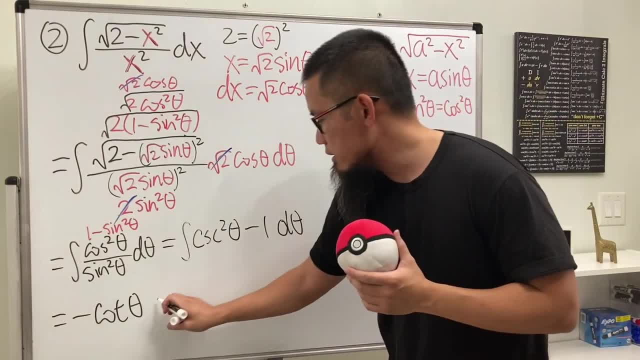 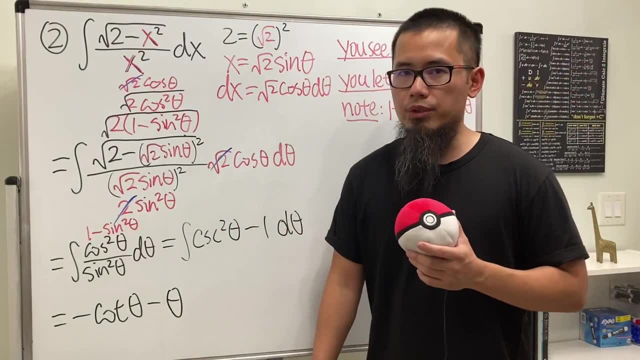 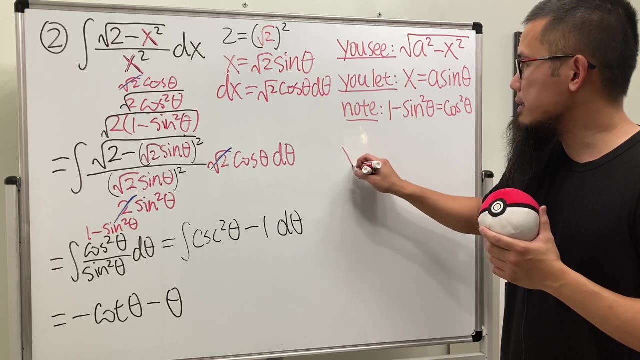 and then minus one in the theta world. integrate that. we get theta right there. okay, now we just have to go back to the x world and this is how. refer back to our substitution right here. i'll put this down right here. we know x is equal to square root of two times. sine theta, we can just: 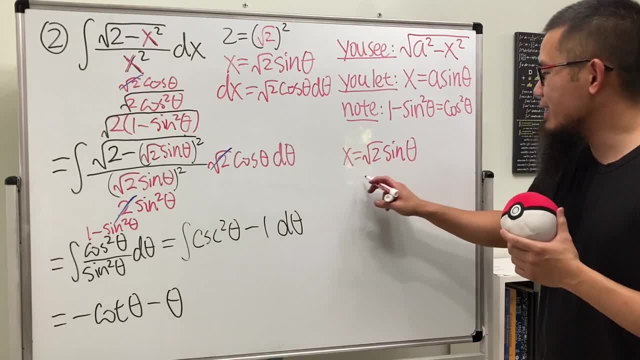 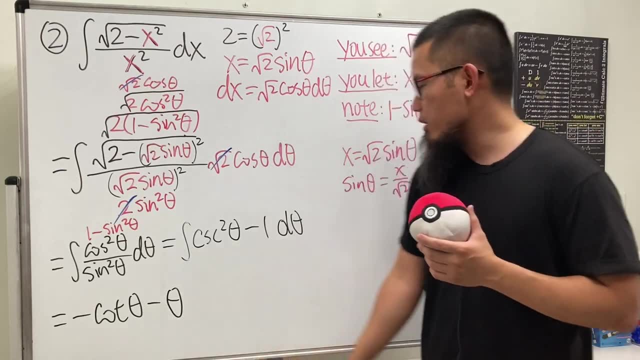 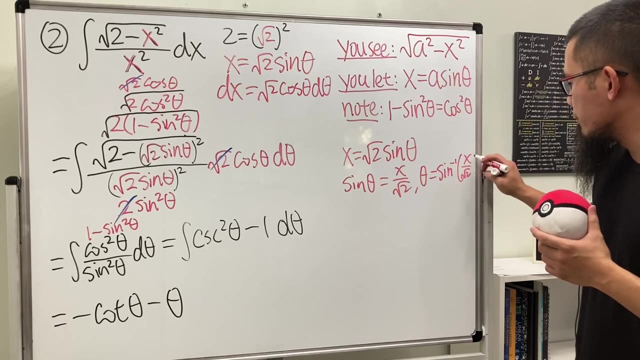 divide the square root of two on both sides, so we get sine. theta is equal to x over square root of two. again, we are looking for the theta here, so theta is just going to be the inverse sine of x over square root of two. so that's okay. well, how do we get cotangent? this is how. so if you look at this, 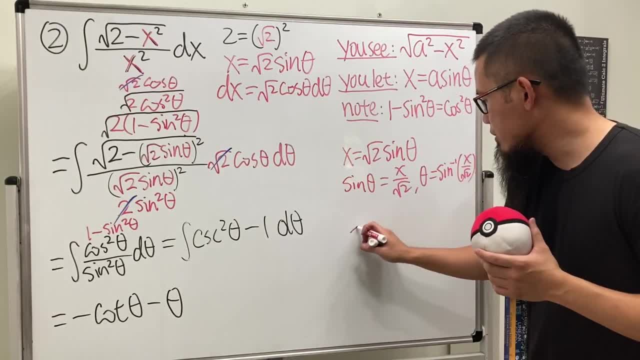 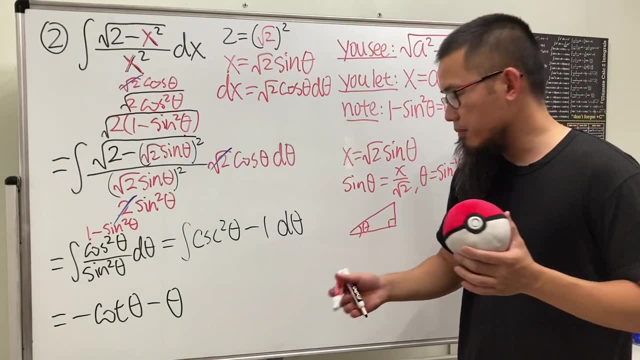 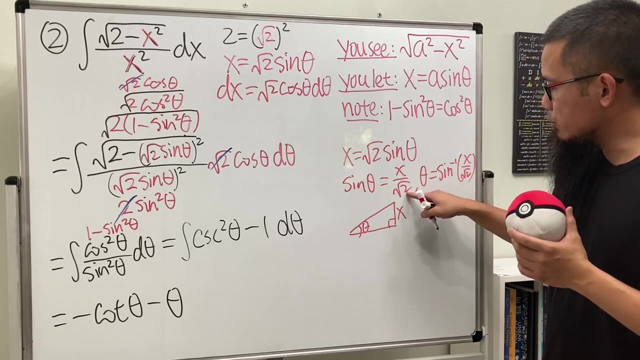 right here we can construct right triangle and i would recommend you guys to always put a right angle right here and the angle theta right here, just to be consistent, because this way you can see x is the opposite, Small Angles, which is right here, and then this right here will be the hypotenuse, because we are talking about sign, so square root. 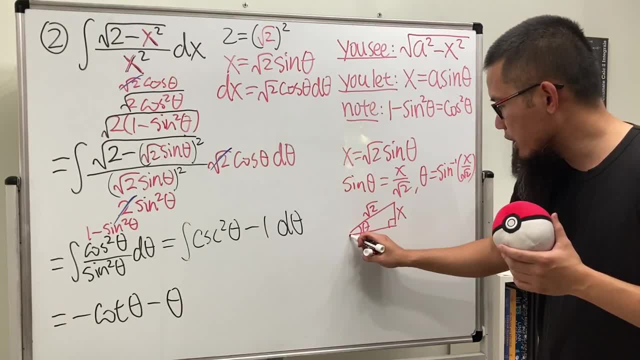 of 2 will go right here and now we just have to figure out the adjacent, and that's going to be. you open a square root, you do this thing square, so square root of two square, and then minus this square and now look at this triangle. we can just do the cotangent. so have a look here we haveLike a square root of two and then minus this square, and now to get this triangle, we can just do the cotangent. So have a look here we have four of those. 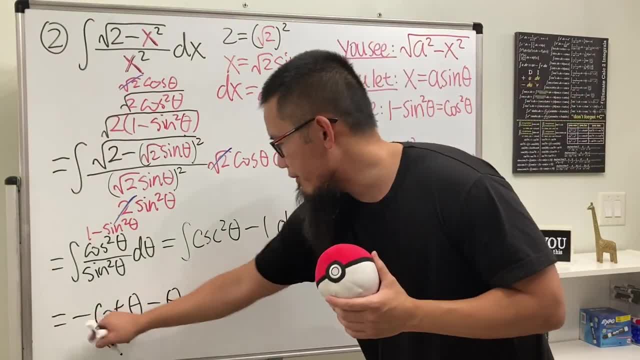 the76.6.6.6.6.. go to the second dot and we can just do the ci tangent. so have a look here. we have a C tangent. so swap Hana and you have 63.13.36.. so have a look here we have negative and for the cotangent is the adjacent over the opposite. 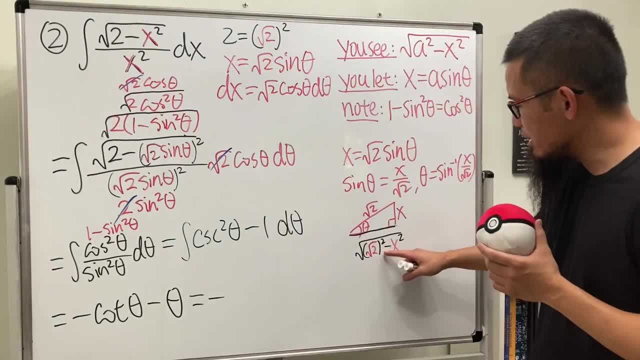 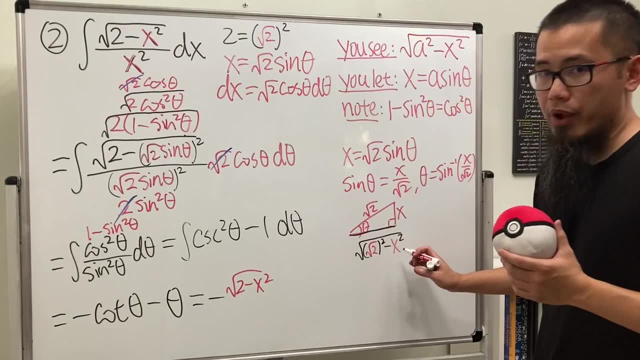 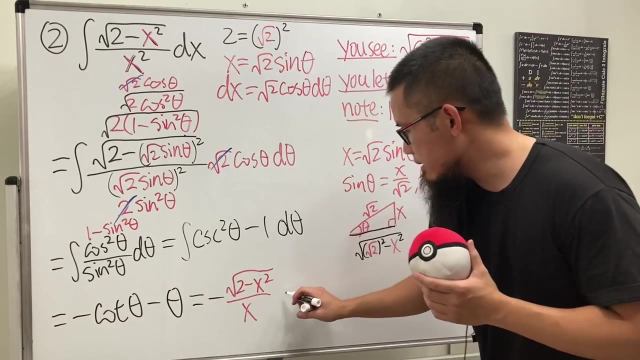 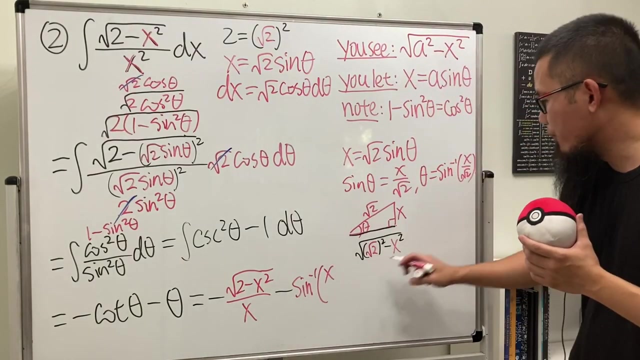 right, it's the reciprocal of tangent. so we do this over that. so we have this, which is square root of 2 minus x square and then over x. so that's what we have, and then minus theta, is this: so we shall done after we put down the inverse sign of x over square root of 2. 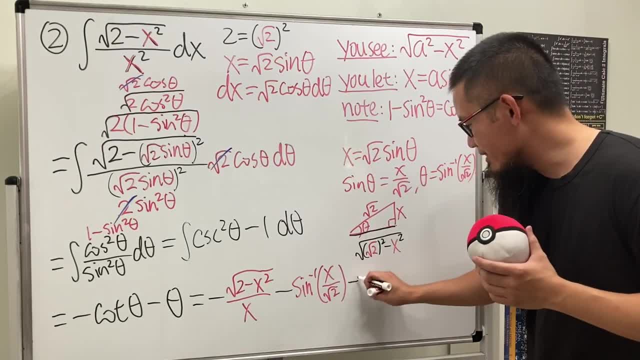 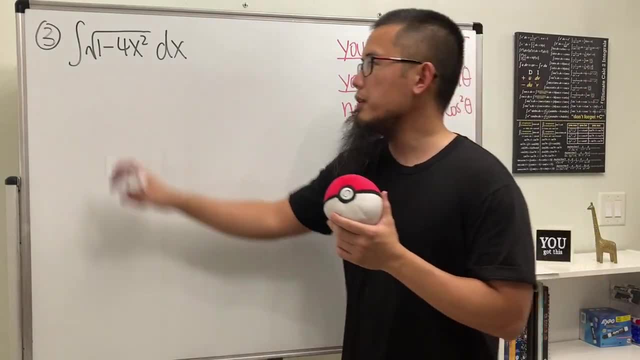 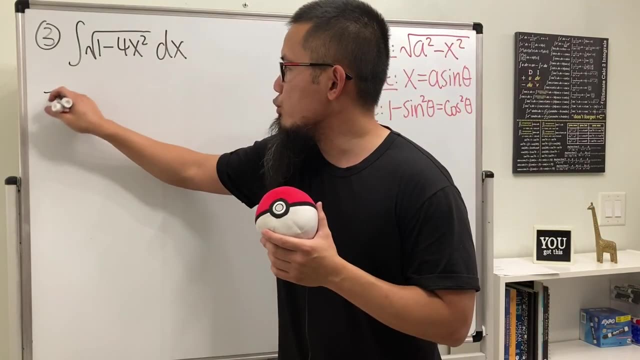 all right. so, of course, don't forget the plus c. this right here is it for number three. we have the integral of square root of 1 minus 4x square, because we have this 4 right here. so this is what we do: we are going to rewrite this integral as the square. 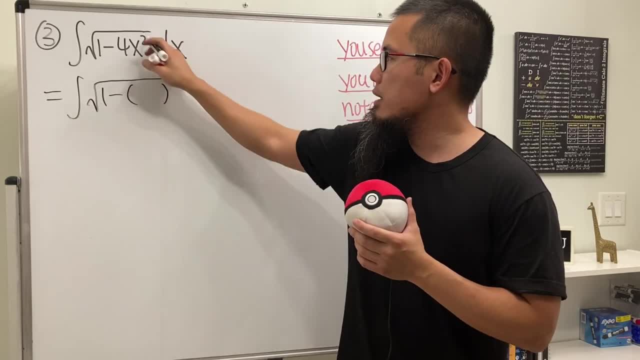 root of 1 minus 4x square, because we have this 4 right here. so this is what we do: we are going to rewrite this integral as the square root of 1 minus 4x square, because we have this 4 right here: minus open. the parentheses make that to the second power. originally: here we have a 4 inside. here we 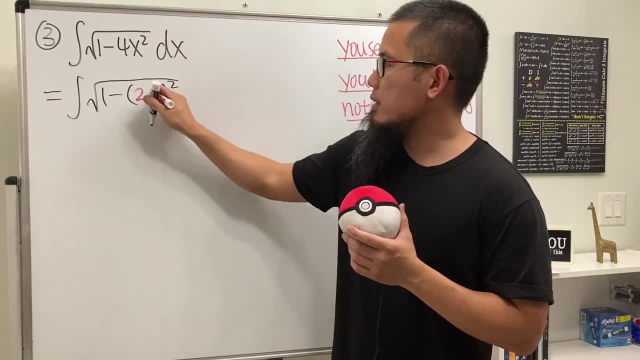 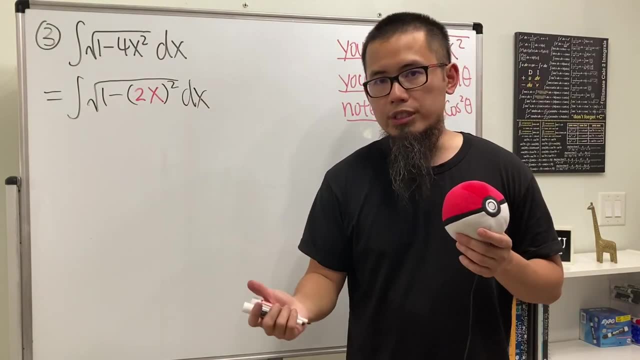 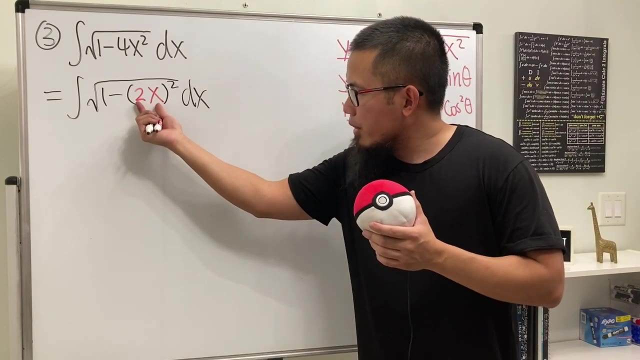 will put 2, because 2 square gives us the 4, and likewise put down the x, right here. and of course we still have the dx. so right here, some people might tell you to do use up, let you equal this and then continue the usual business. but i will tell you, you see this, right here, it will be the 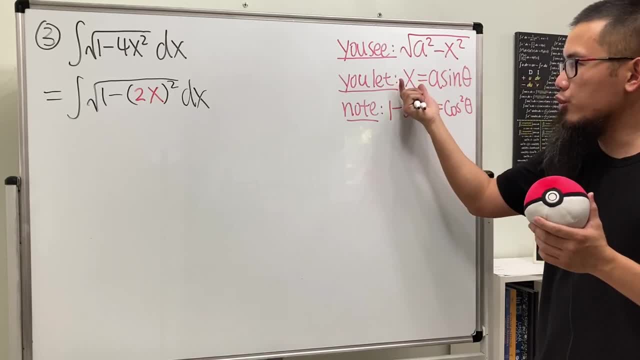 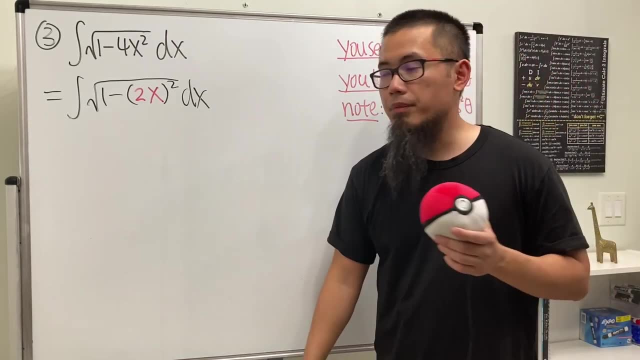 new x square part right here, and then we will put down the x right here, and then we will put down the x right here, and then we will put down the x right here, and then we will soap here, and it's just going to be that we are going to let this the 2x equal a times sine theta. that's all and notice. 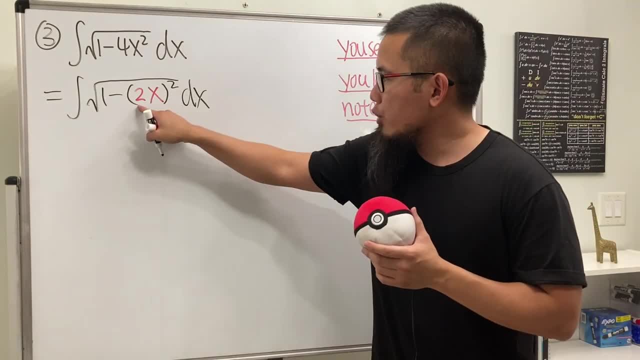 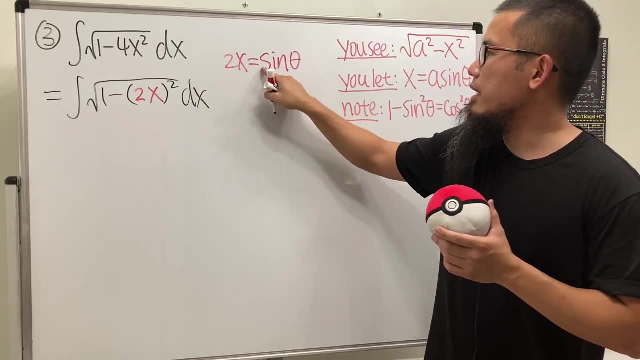 that a is equal to 1, so i'm going to just do it that way. i think it's pretty clear. so right here, i'm going to put this right here, which is the 2x: make that equal sine theta. again, our a is equal to. 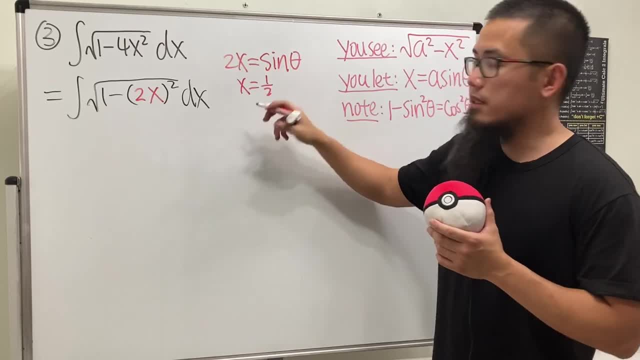 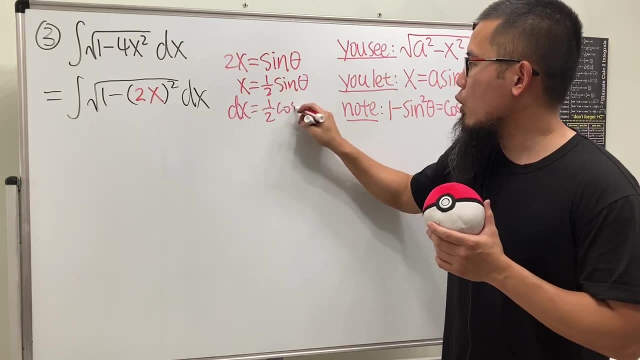 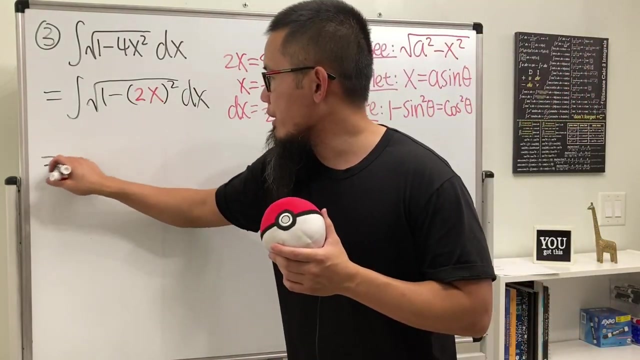 one. once we have this, we can divide the two on both sides before we differentiate, and we'll just so. x is equal to one half sine theta, and then dx is equal to one half cosine theta, d theta. so now we can take this integral to the theta world and we will get the integral, and then we 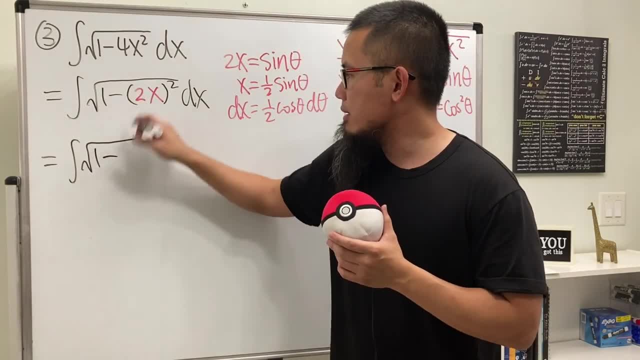 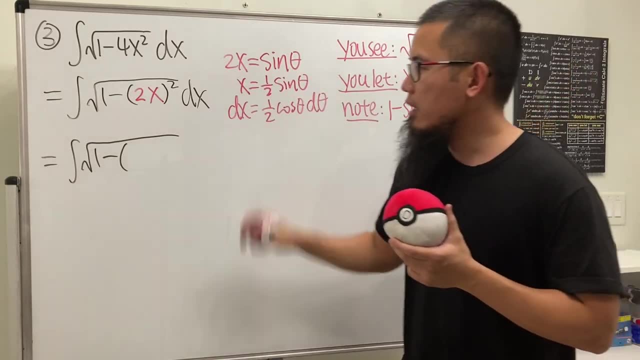 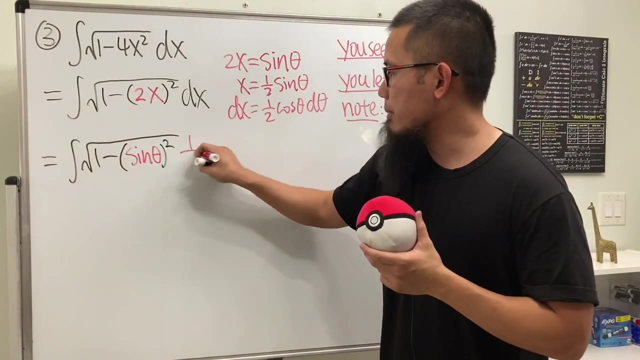 have the square root. one is one minus parentheses, the parentheses. and now we see, inside here we have two x and that's exactly what we said to be the sine theta. so i can just replace that right here, and then we have to square that and then the dx is all that. so multiply by one half cosine theta. 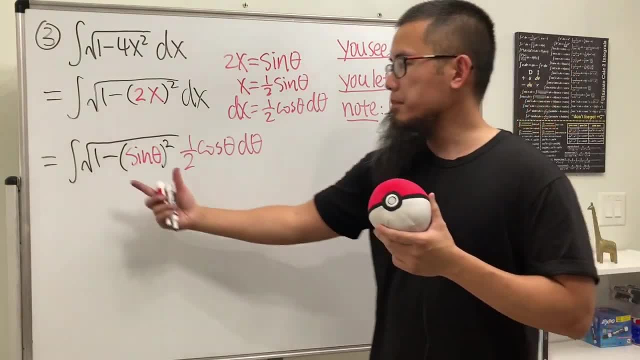 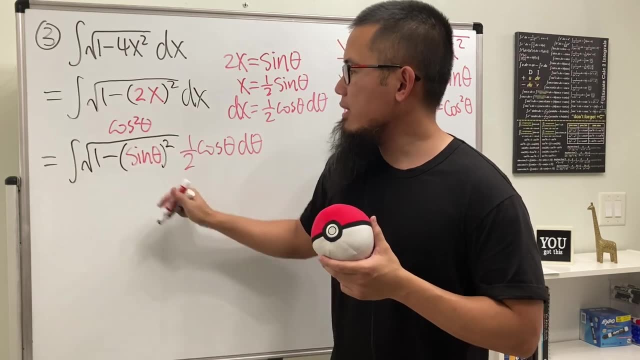 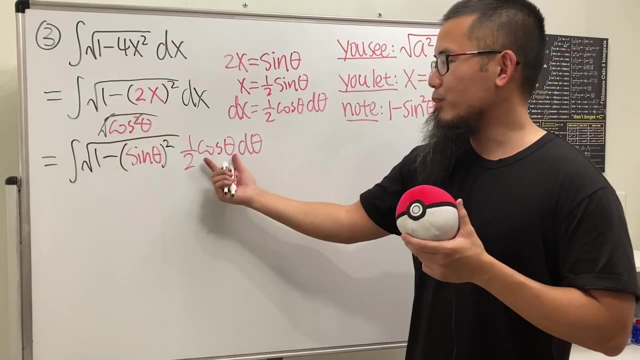 d theta. okay, now we have to simplify this. one minus sine squared theta is just cosine squared theta, and then we have to take the square root for that, but again this and that will cancel. so we just have cosine to the first power and we have to multiply by another cosine to the. 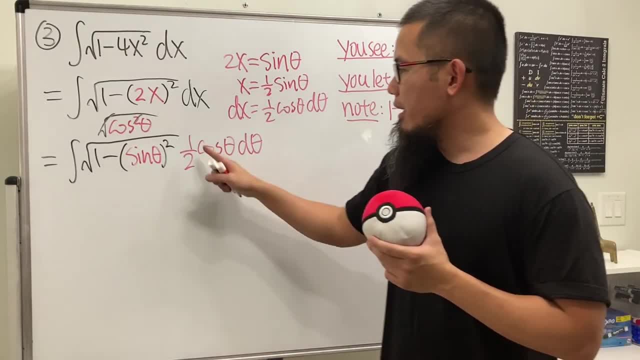 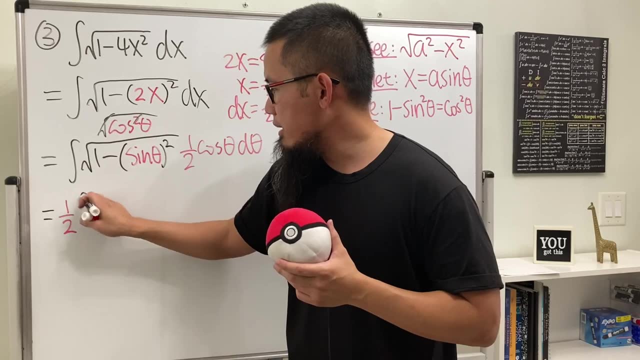 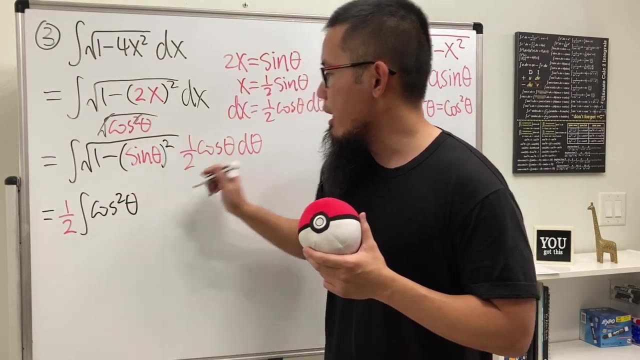 first power. so that's cosine to the second power. you here, we have one over two. let's put that in the front of the integral. and then we're looking at the integral, cosine x: well, cosine theta times, cosine theta, as we said, that's cosine square theta. and then we are in the theta world, like this: 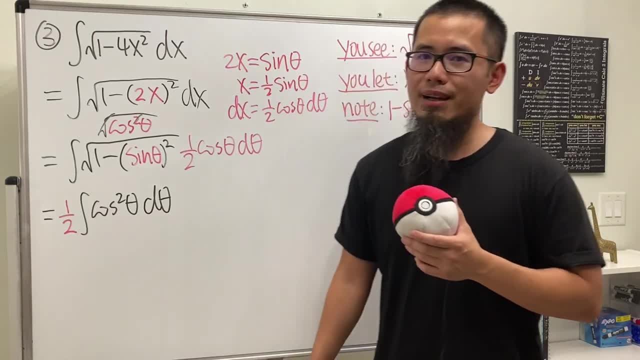 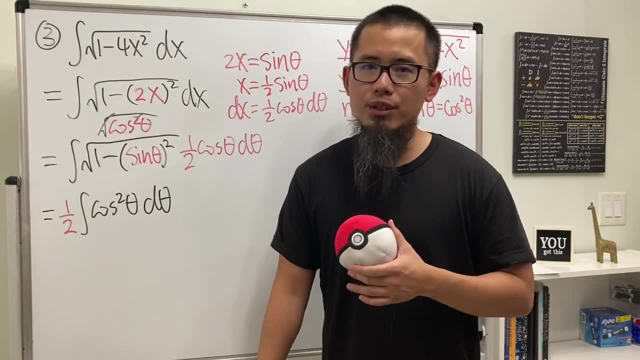 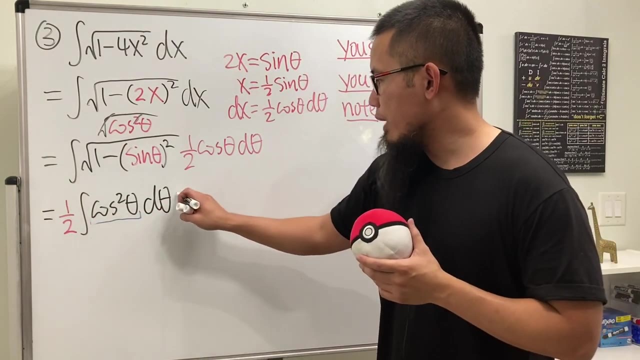 well, well, how do we integrate cosine square theta? we will have to use the identity, right? we don't want to have cosine to the second power, we want to have cosine to the power. All right, this is the identity that we are going to use. I'm going to first write down: 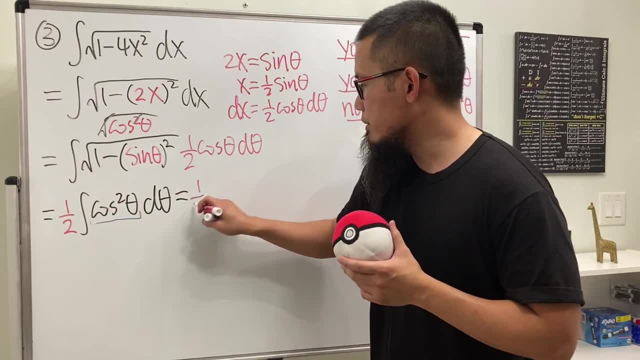 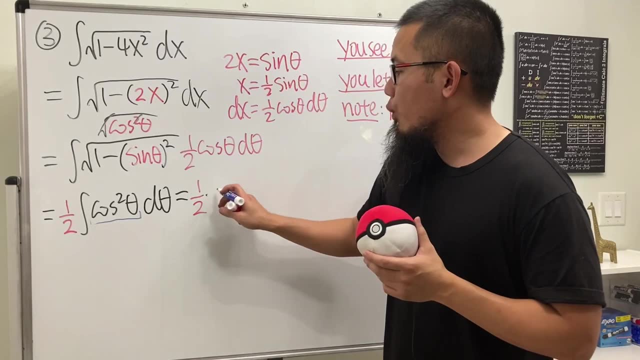 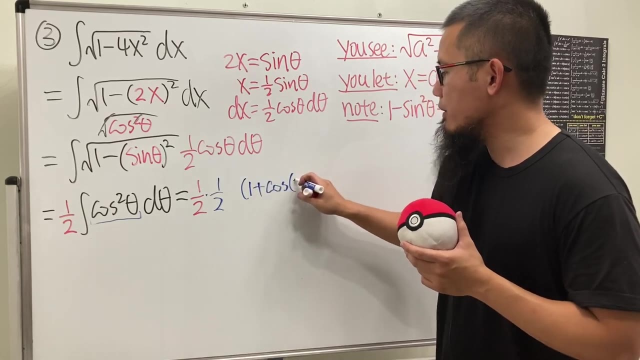 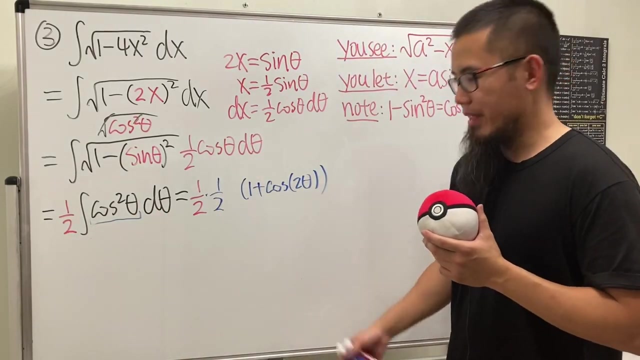 the 1 half in the front. so this right here doesn't change from here. However, the identity for cosine squared theta is 1 half, and then we multiply by 1 plus cosine of 2 theta. So the blue part is for that. so that's why we have another 1 half, And then we still have to integrate that. 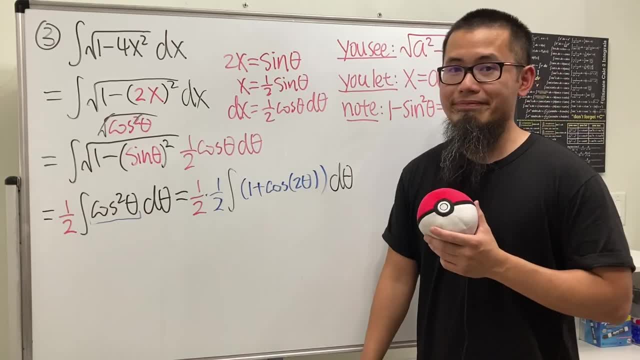 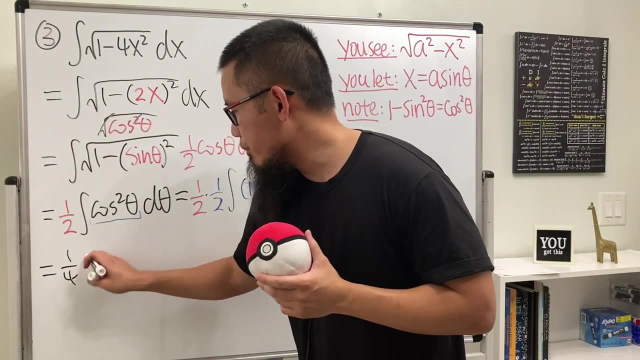 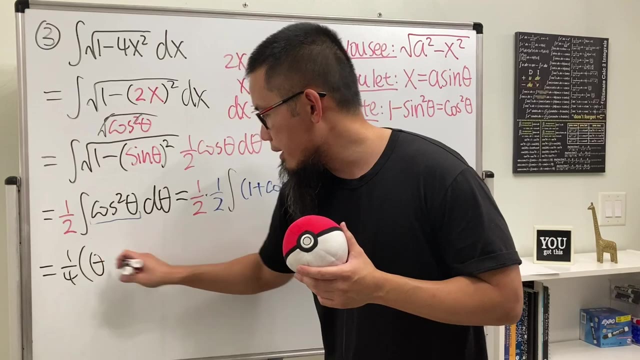 and then this is still in the theta world. Okay, now, this times that is of course 1 over 4, and then I'm going to open the parentheses for the result of integration: 1 in the theta world will give us theta, and then, integrating cosine, we get positive sine. 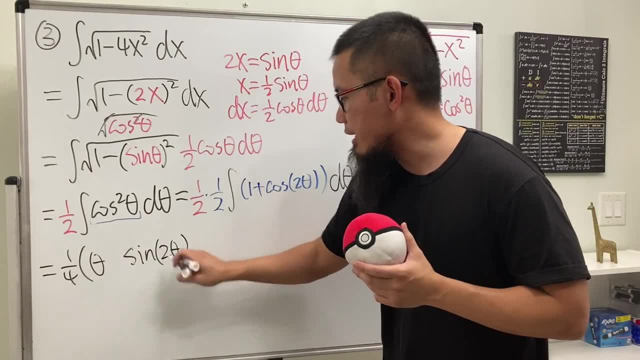 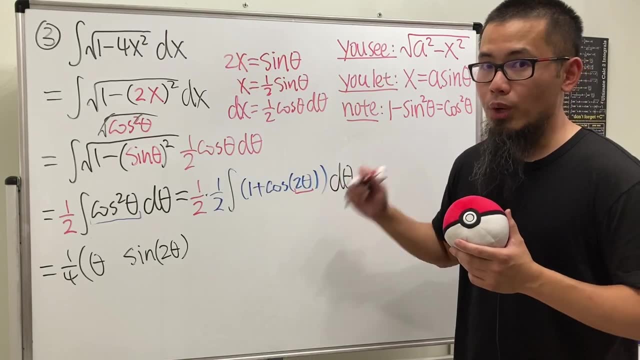 and then the input states the same, which is 2 theta. And again, because the derivative of 2 theta is just a 2, so we can do this And, of course, don't forget that we will have to divide it by the derivative of 2 theta, which is 2.. I'm going to be putting down 1 half right here. 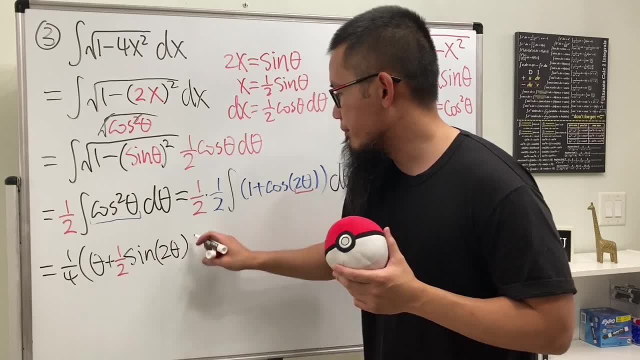 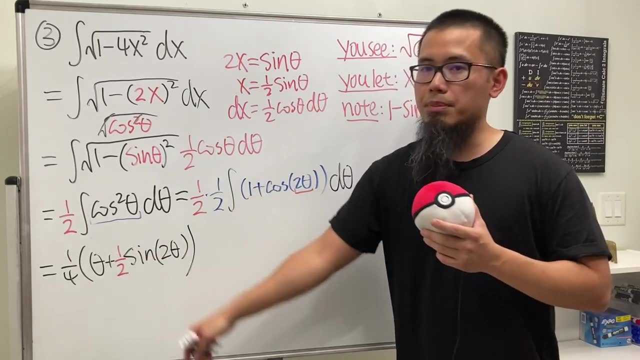 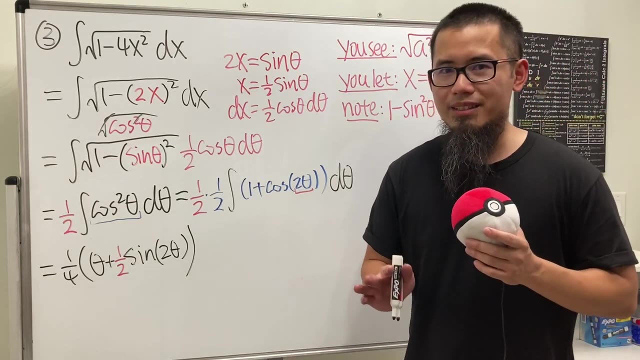 and then we can just put down a plus right here, because the derivative of, because the integral of cosine, is positive sine. so that's why it states positive. so just like that, All right. I know this is a lot of work, but we're not done yet, We're almost done, all right. 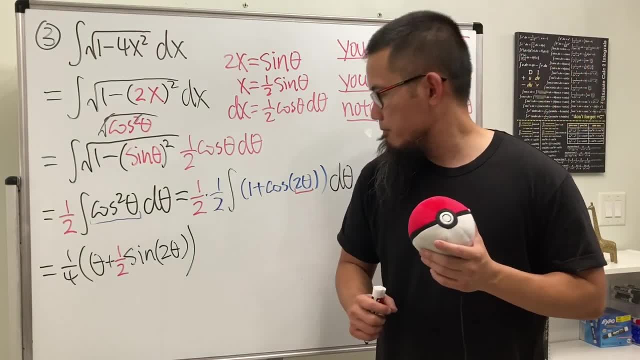 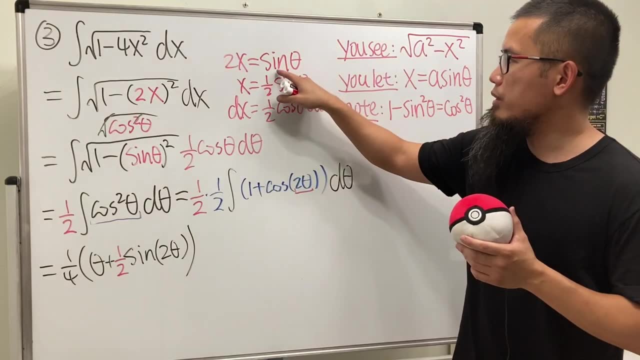 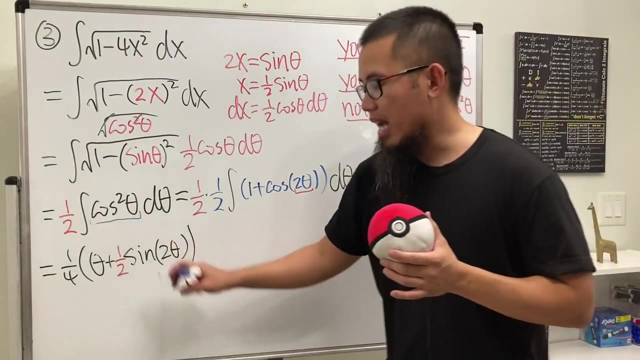 Again, we will have to go back to the x world. But the problem here is that here is sine 2 theta. Our original substitution only deal with theta inside, so we will have to do the double angle identity for sine, This part, right here. 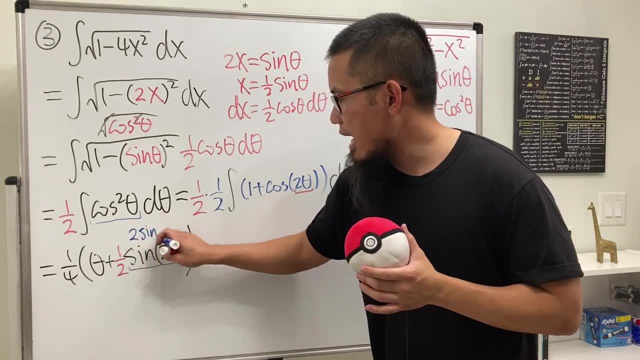 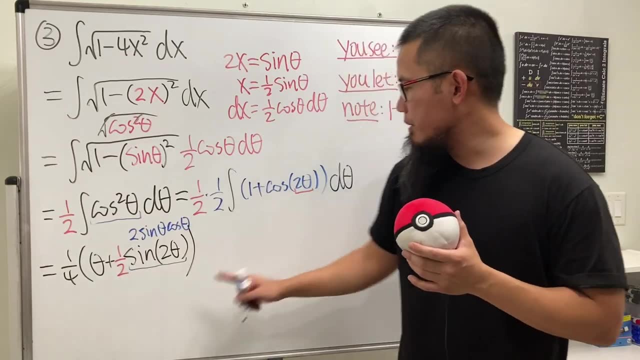 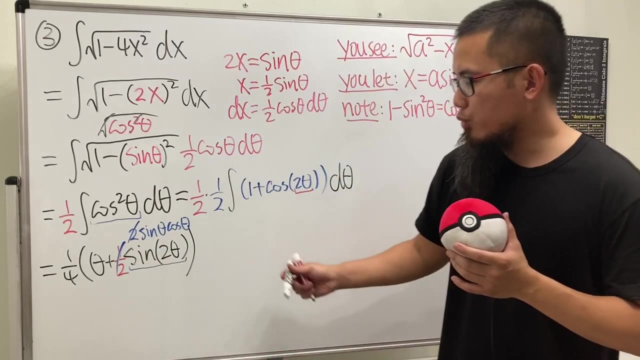 is the same as 2 times sine theta and cosine theta, And you see, here we have the 1 half, because from here, 1 half times this 2, well, they cancel each other out. So I'm going to write down what we have. 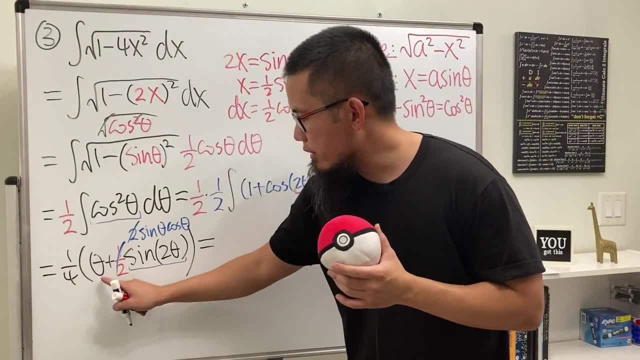 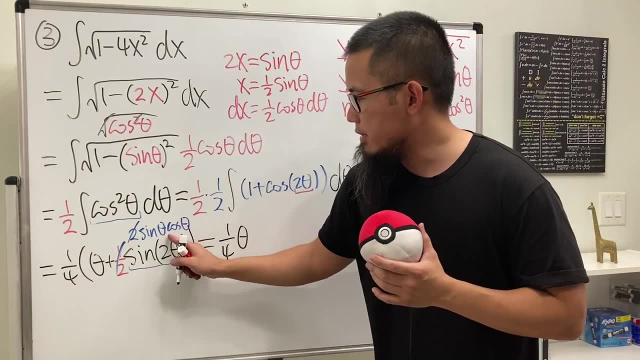 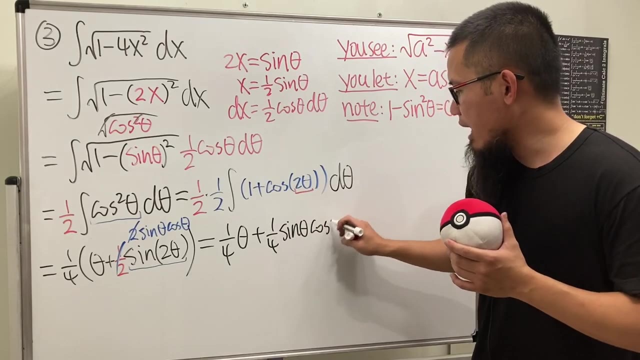 right here for you guys: 1 over 4 times theta, so that's 1 over 4 theta. Next, 1 over 4 times this, which is just plus 1 over 4, cosine, theta, Cosine, theta. So that's what we have. So that kind of clears up the constant. 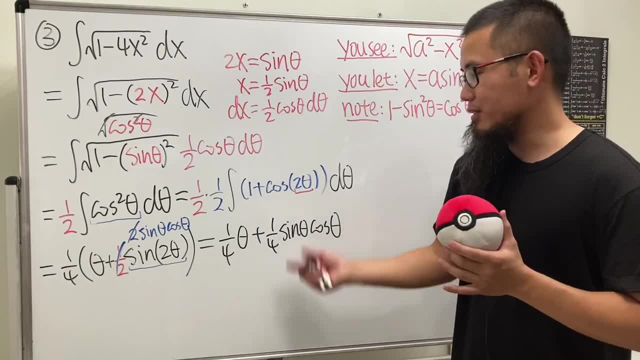 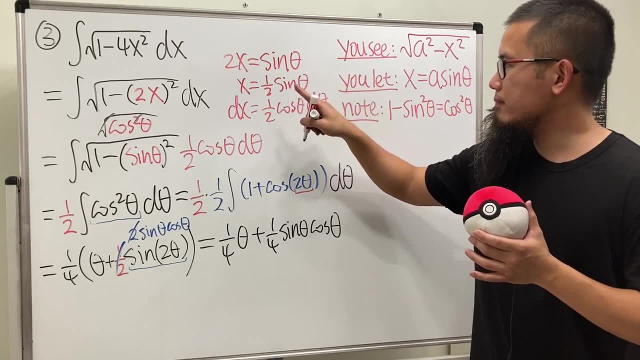 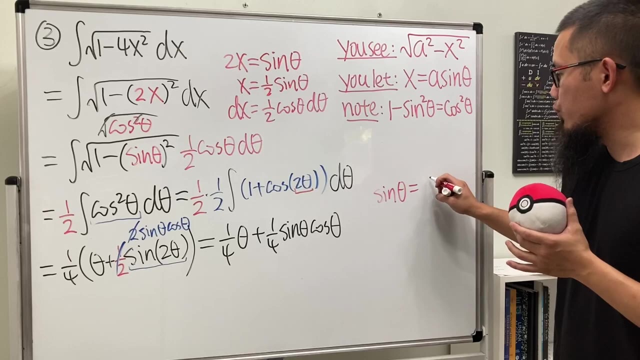 multiples, and I think we're okay now, And the final step is go back to the x world, as we said earlier. Well, let's see We are going to look at. look at this right here. Look at this: We know we have sine theta being equal to 2 x. 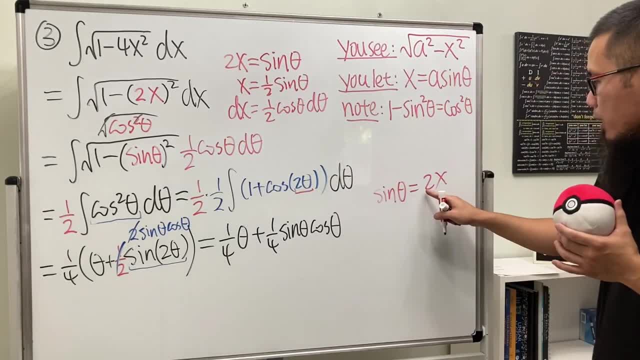 This can be done with more than one time derivative outside, because you're using only time. Isn't it pretty easy to look at the Runner of R To 2500 and 500 medicine? Because, if you, though, i'm going to purposely look at this as 2x over 1, because we are going to construct 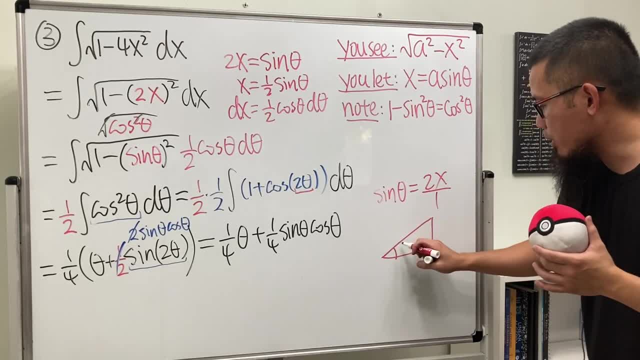 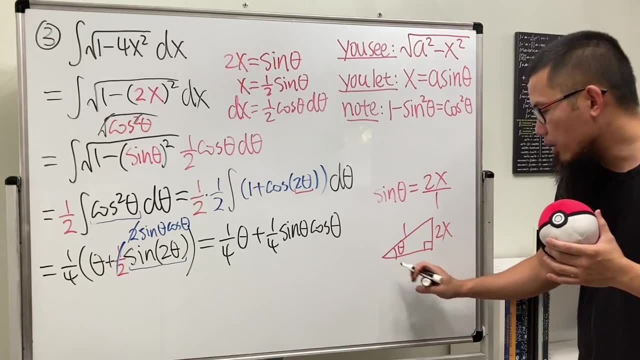 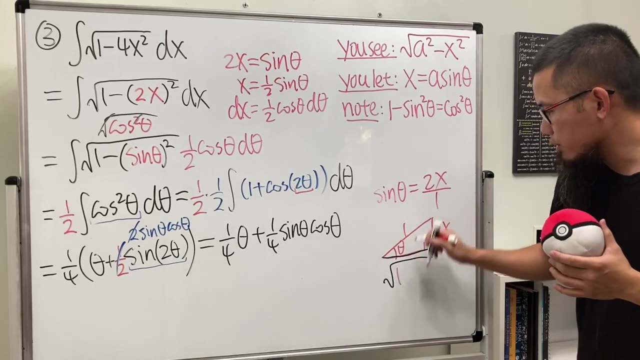 a right triangle, put the right angle here and then the angle theta here sine is opposite over hypotenuse. so now we are going to figure out the adjacent which is square root, this thing square. so be sure you do the hypotenuse square first and then minus. 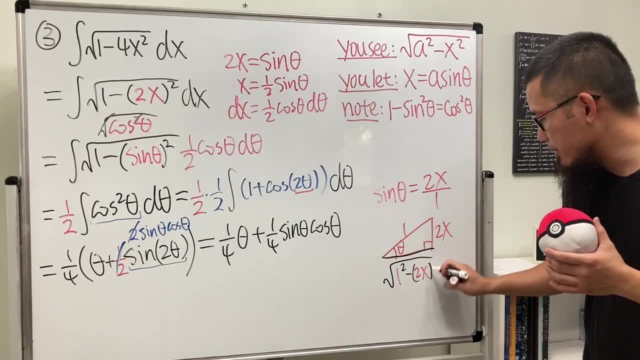 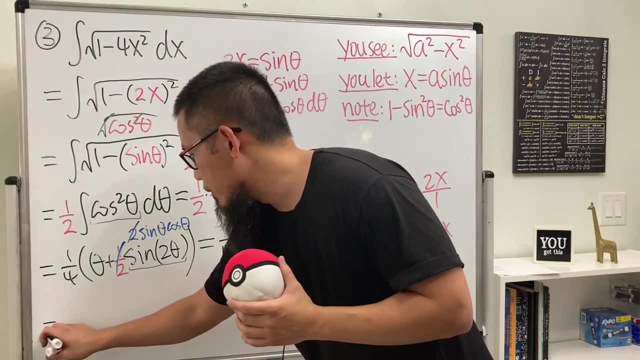 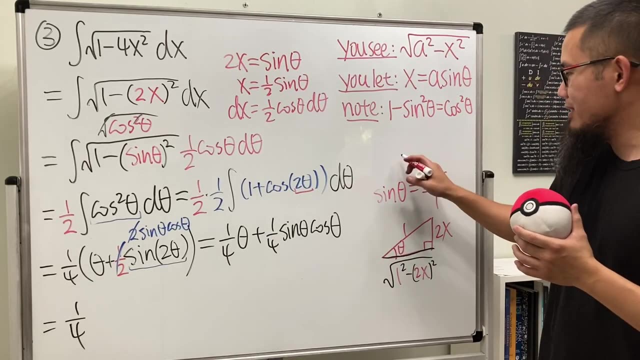 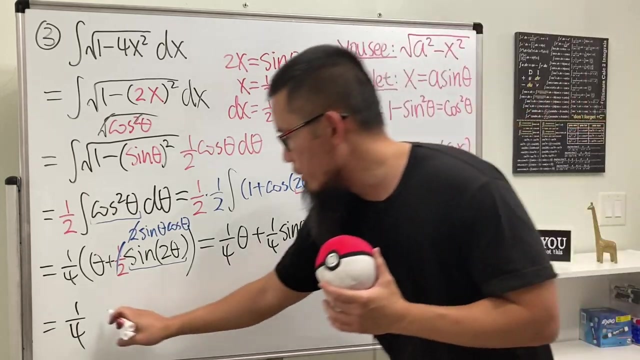 this thing square, so we'll have the 2x and then square. so this is pretty much all we need. let's go ahead and figure this out. so here we see that we have 1 over 4. theta is just going to be the inverse of 2x, right, so we can just put that down. we have the inverse sine of 2x. so that's the first part. 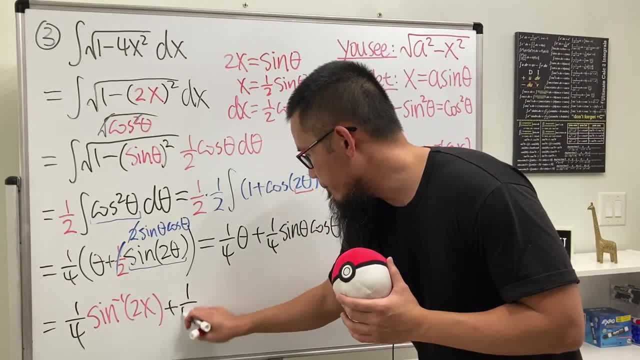 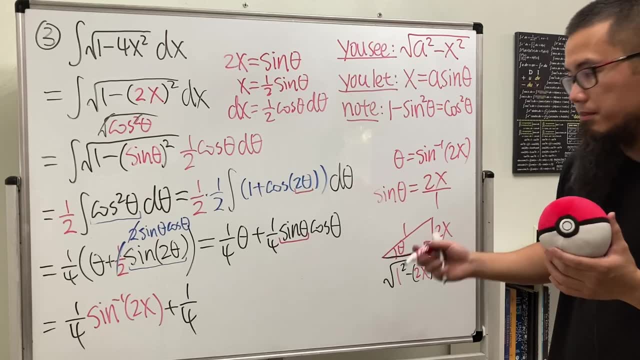 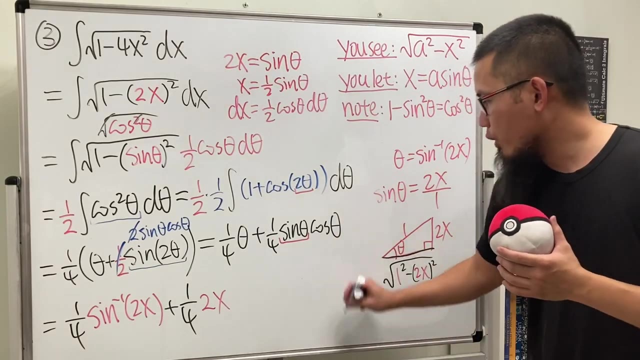 next we have plus 1 over 4 from here, and then sine theta is the 2x, right, sine theta is just the 2x, so we can put that down right here. next we have cosine theta. well, for cosine theta, here we can look at this triangle and cosine is: 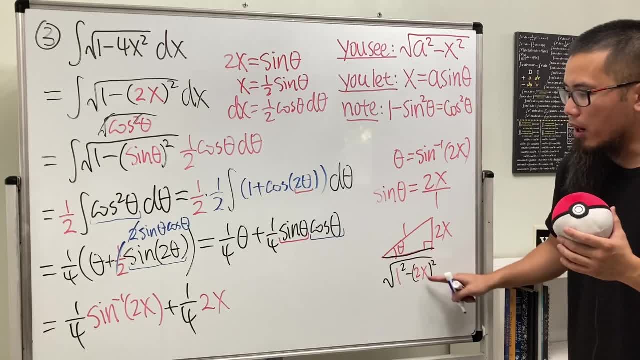 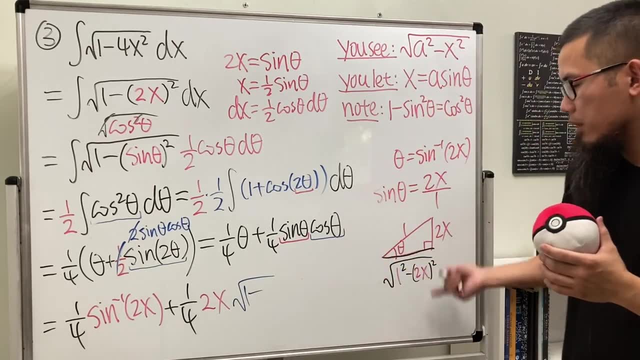 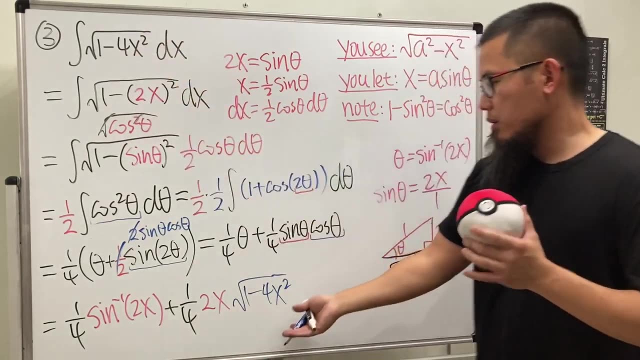 adjacent over hypotenuse, which is just the square root part, and that's going to be square root of 1 minus 2 square and x squared right. so it's just 4x squared and of course you can kind of expect that the original square root part you know appears again. so that looks pretty good, yep. 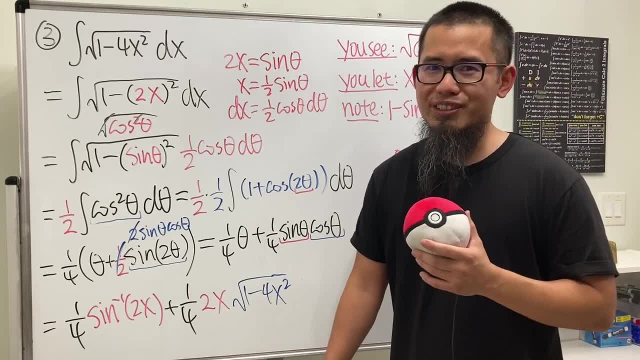 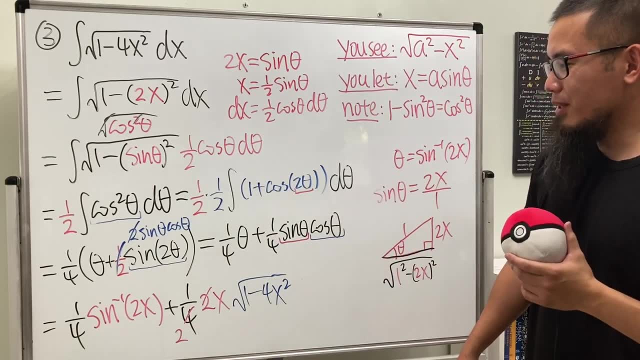 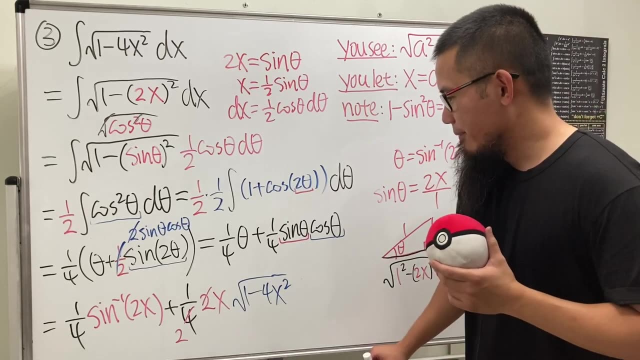 so that's pretty much it, but of course, the final touch is that i'm going to reduce this a little bit. so yeah, that's pretty much it, and perhaps i am just going to erase this triangle. uh, i don't know, because you see, this is the problem. sometimes you just write. 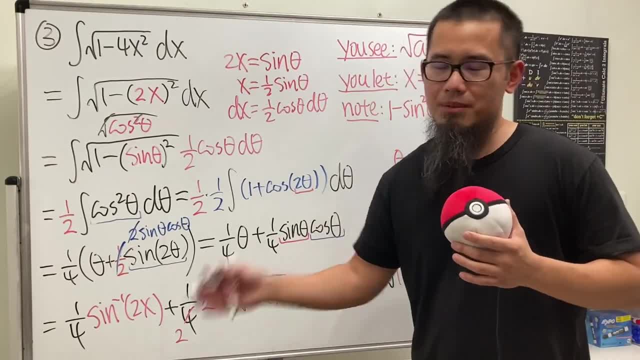 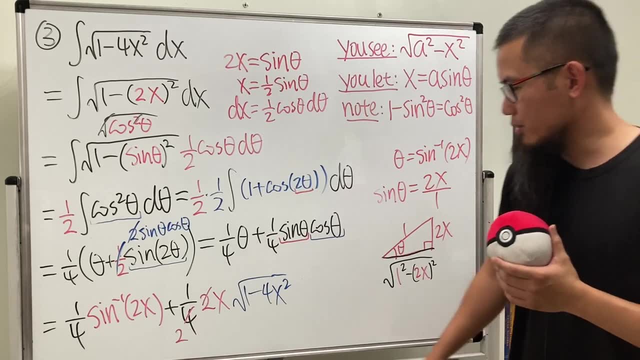 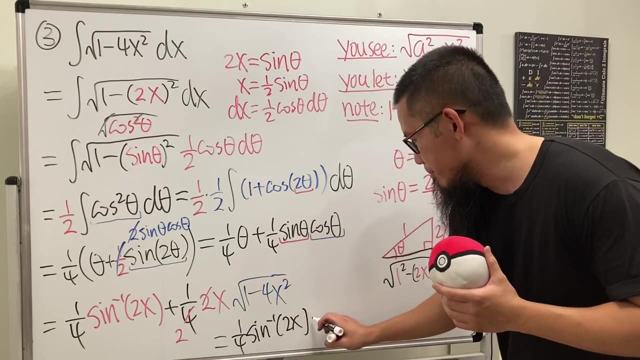 down the same thing over and over again. if you leave this on the test, my students, i will be totally cool with that, right, you don't have to copy down the same thing over again. but, um, i'm making a video, so i'm going to write this down one more time: 1 over 4, inverse sine of 2x and then plus 1 over 2. 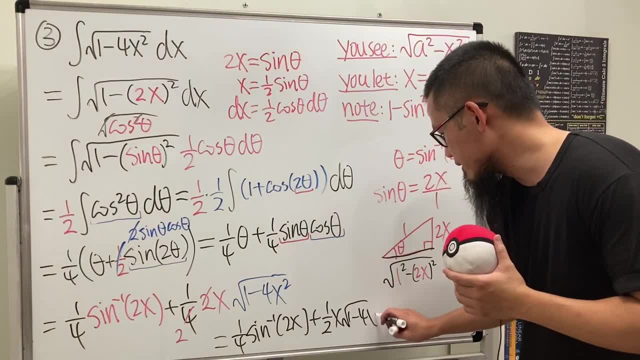 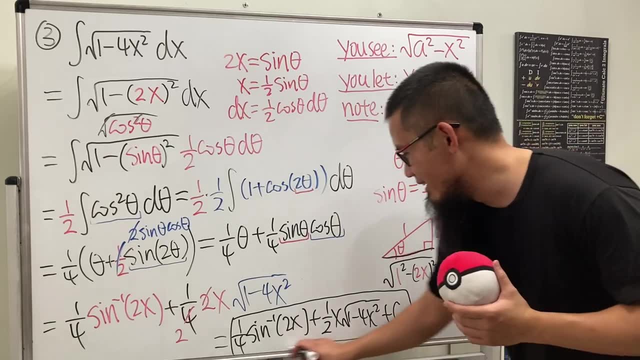 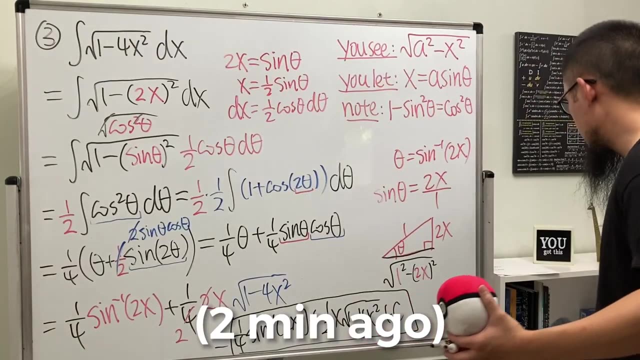 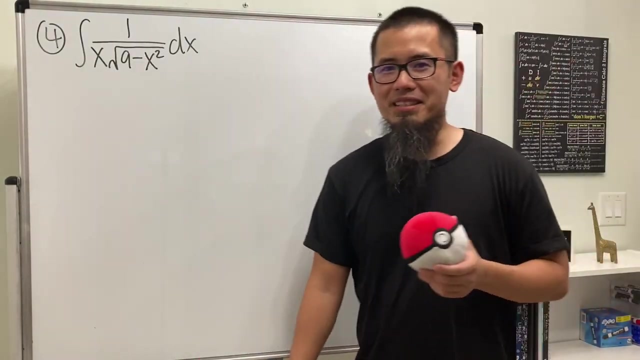 x square root of 1 minus 4x squared. and then we are all done. so. here will be the answer for that. okay, i accidentally erased the notes right here, but it's okay. this is number four already. here we have to integrate 1 over x times the square root of. 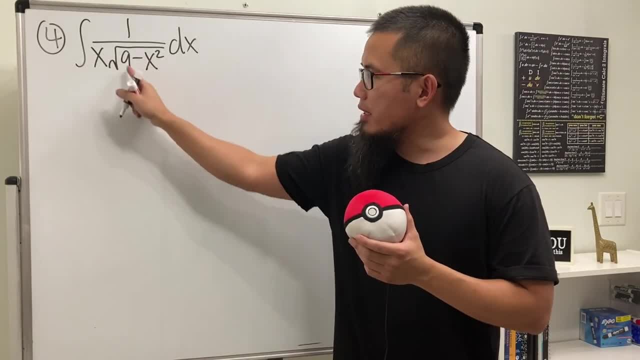 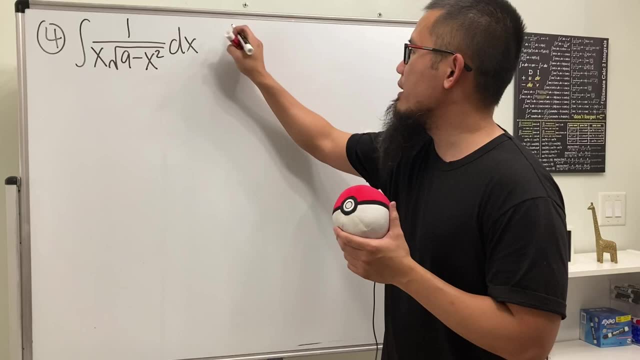 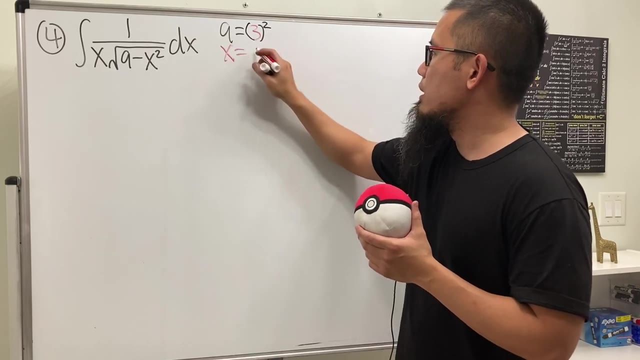 9 minus x squared. so focus on inside of the square root. this is the 9. well, that means a is equal to 3, so let me just write that down real quick: 9 equals 3 squared. all right, so we are going to let x equal 3 times sine theta and then do the usual business. 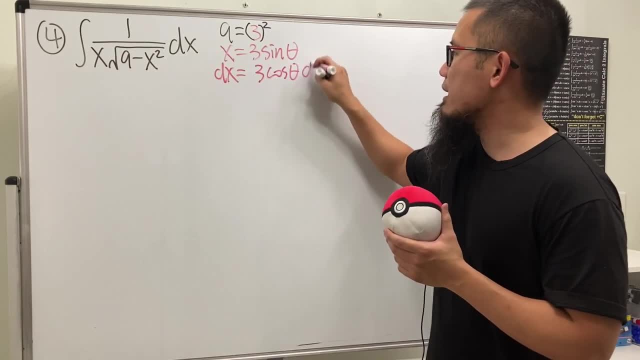 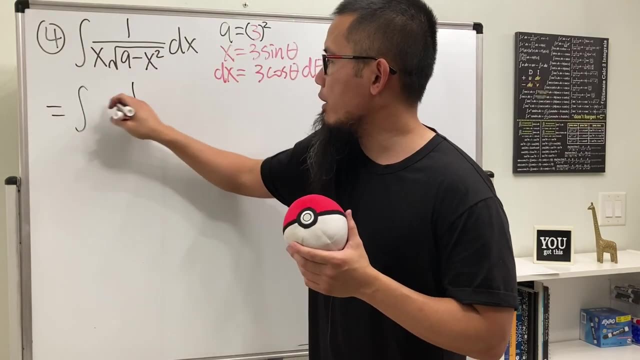 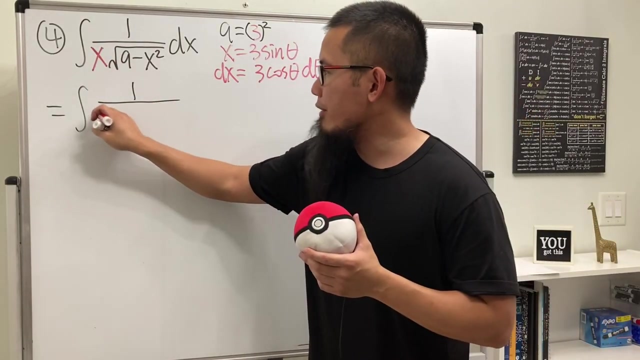 dx is just going to be 3 cosine theta, d theta. and again, take this integral to the theta world. we are looking at the integral of 1 over here. we have this x right here, which is 3 sine theta, so we have to put that down and then we have the square root. 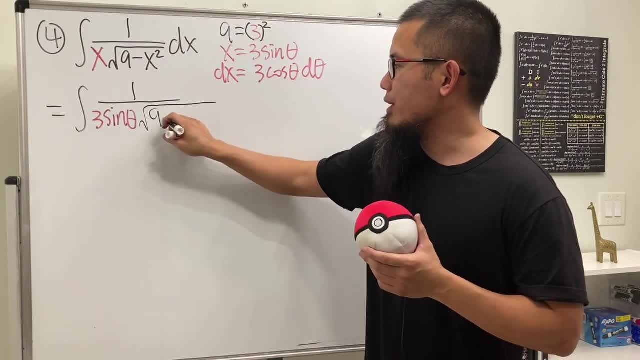 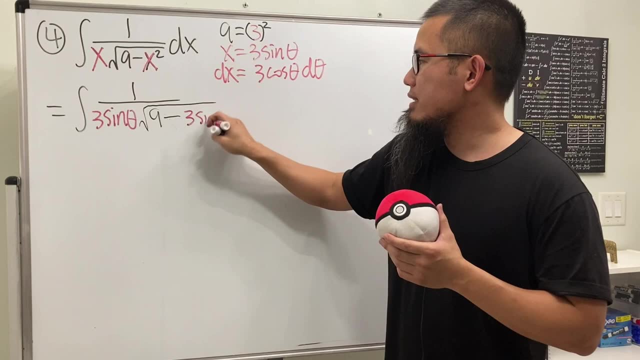 9 minus. oops, didn't write it well. here we have x squared x, is that so? write down 3 sine theta, and then we will have to square this. here we have x squared x, is that so? write down 3 sine theta, and then we will have to square this. 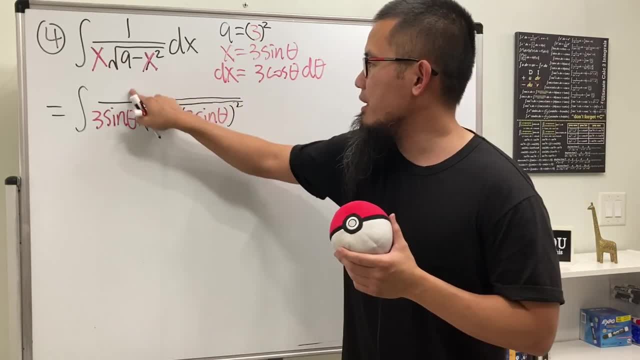 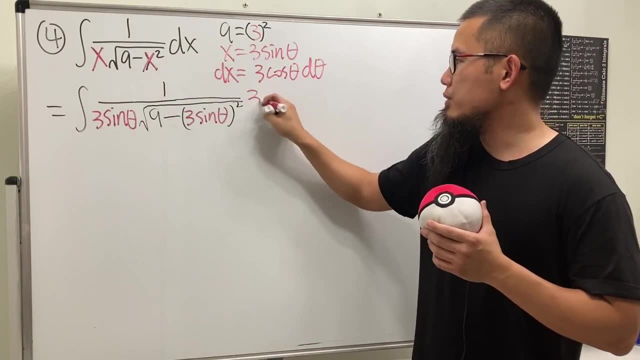 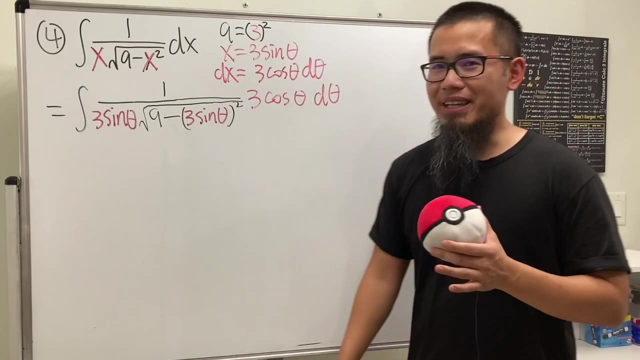 yeah, I know another big expression, but don't forget, for the dx, we also have to put down this right here. and that's 3, cosine: theta, d, theta. wow, I know. okay, simplify this part right here real quick. this is 9,, this is also 9,, so we can factor out the 9, and then multiply by. 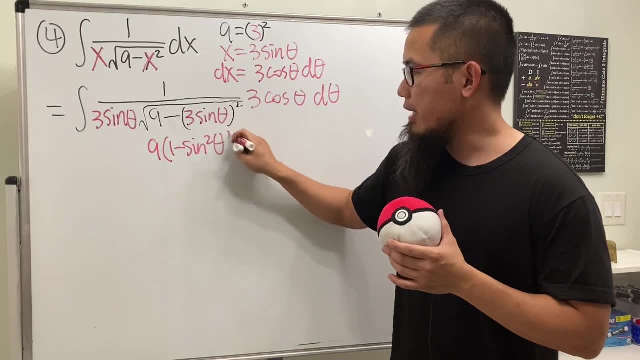 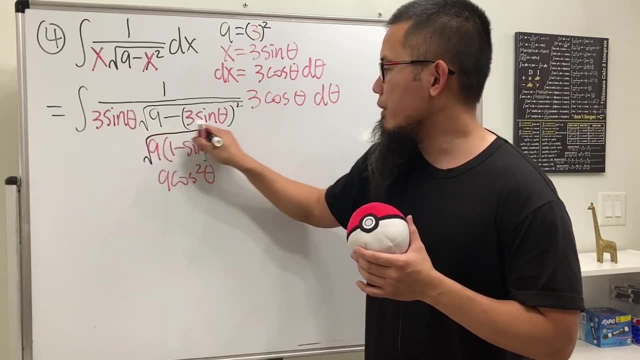 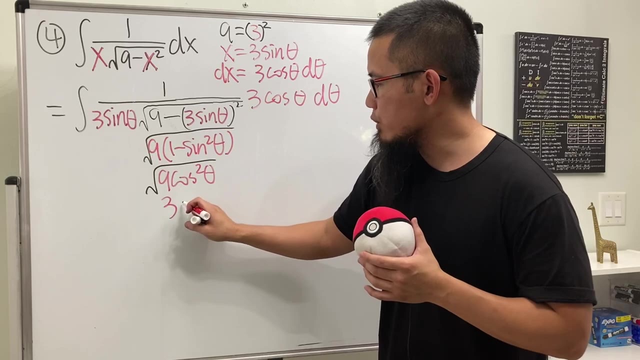 1 minus sine squared theta. this right here is just cosine squared theta and we have the 9 in front again. these two things right, they are still in the square root. this will give us just the 3, and then cancel out the square root, so we have cosine to the first power theta. 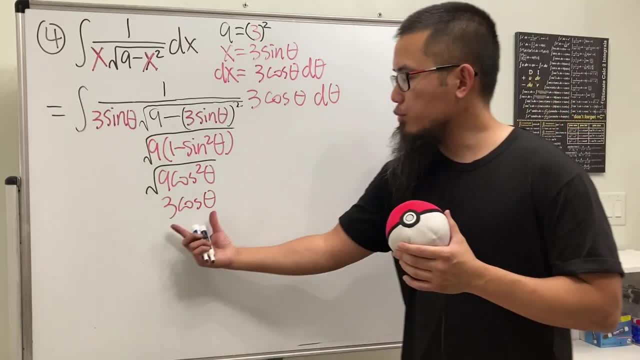 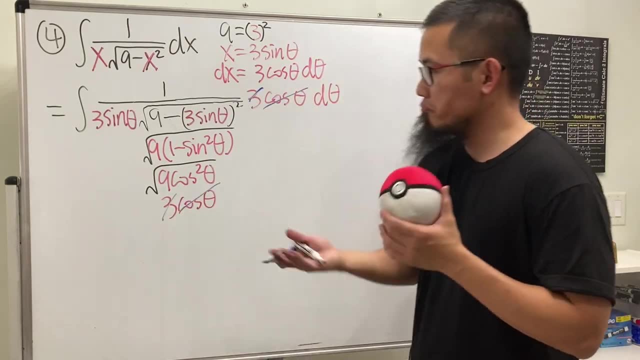 so that's what we have. okay, notice that this right here is on the bottom and this right here is on the top, so we can actually cancel, cancel and likewise cancel, Cancel, cancel. pretty good, pretty good, I would say. so what exactly are we integrating? 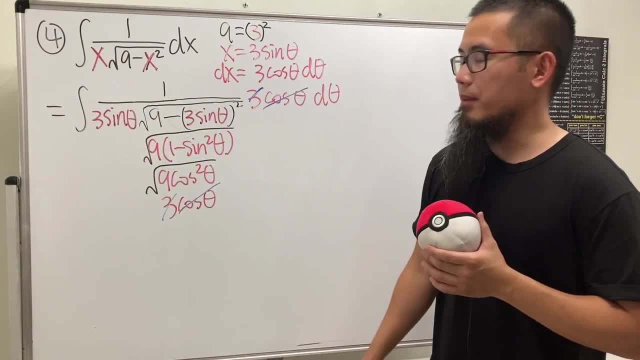 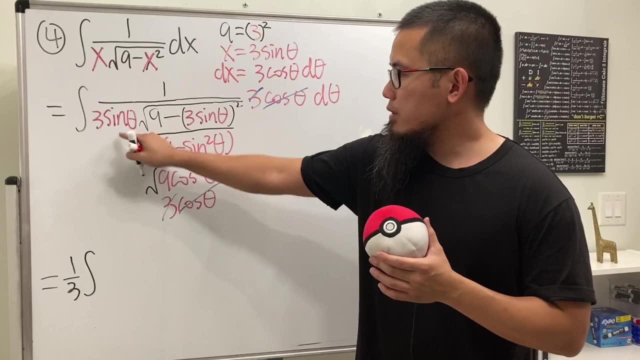 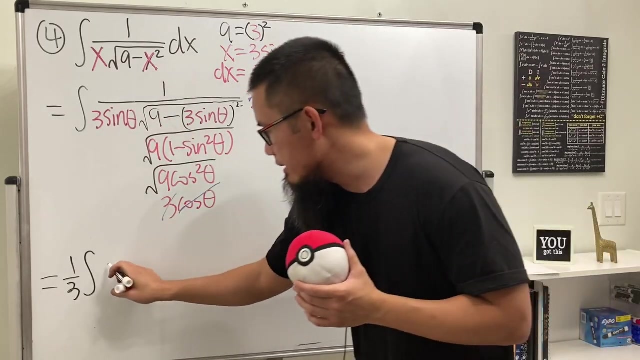 Well, this right here is just going to be 1 third. and then we have the sine theta on the bottom and I'm just going to write it down right here: 1 third integral. because we just have 1 over sine theta, they are gone. 1 over sine is cosecant, so let's put that down right here. 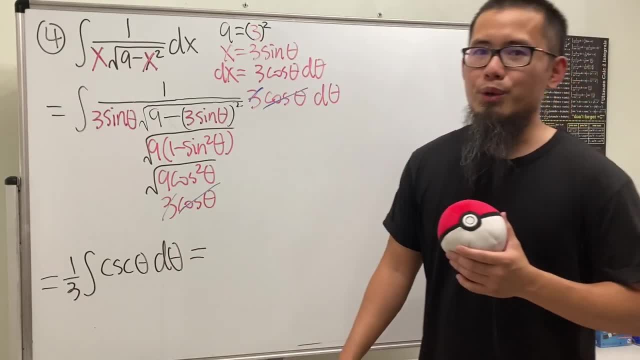 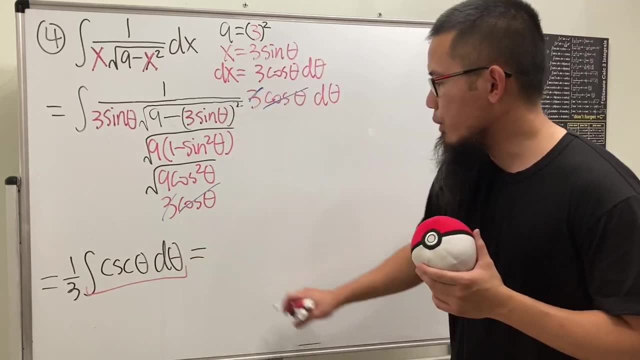 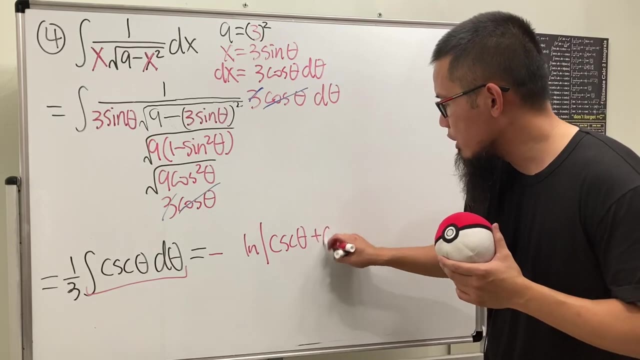 okay, how do we integrate cosecant Cosecant theta? this is a standard result, so you have to remember that. here's the deal. this right here is equal to negative ln absolute value of cosecant theta plus cotangent theta. 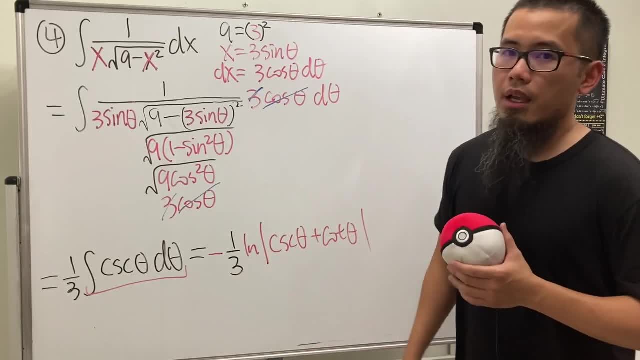 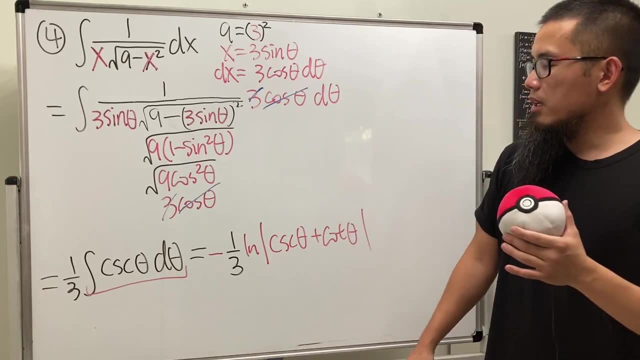 and of course we still have the 1 third right here and I want to make this clear: if you look at like some textbooks, or maybe if you look at some notes online, some people might say the integral of cosecant theta. 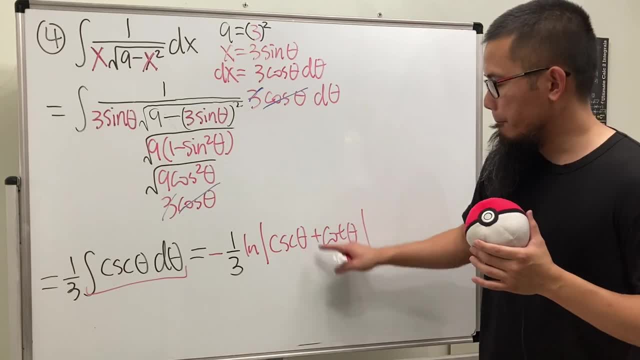 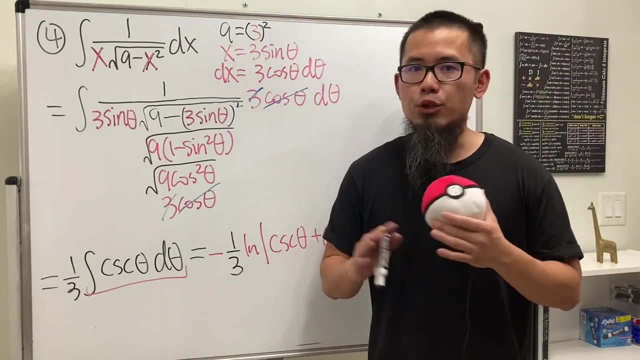 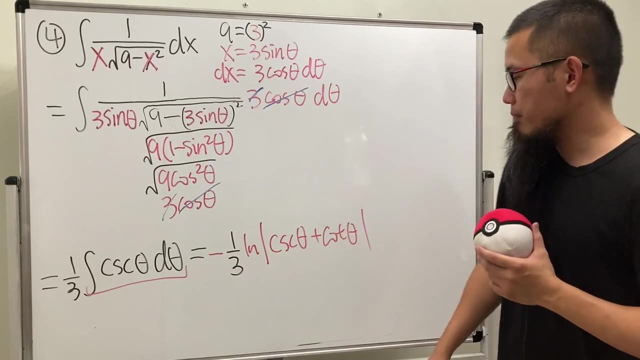 is ln absolute value of cosecant theta minus cotangent theta. they have the minus instead of right here. they have it here. in fact, they are equivalent identities, so this one, or if you have the negative right here, yeah, okay, but I have a video going from here to here so you guys can. 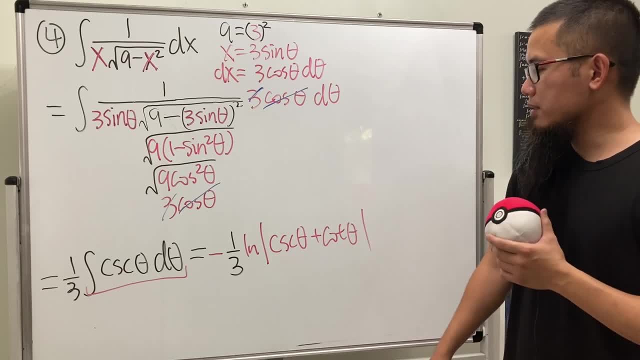 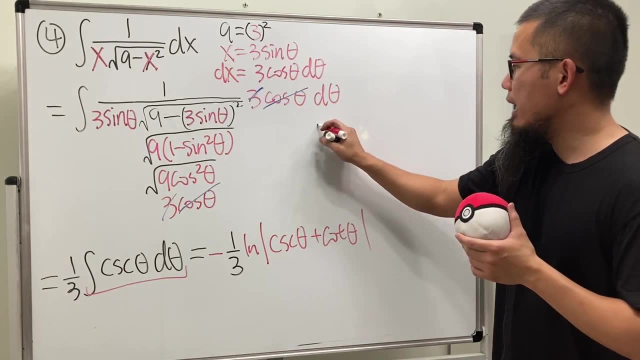 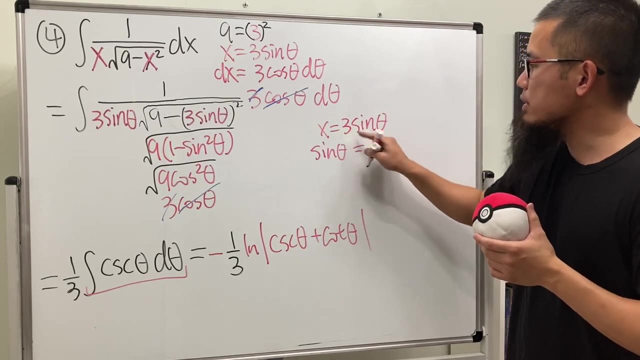 check that out. okay, so now the usual business is just that we have to go back to the x world and we'll be done. Look at this right here real quick. we know that x is equal to 3 sine theta. this means sine theta equals. 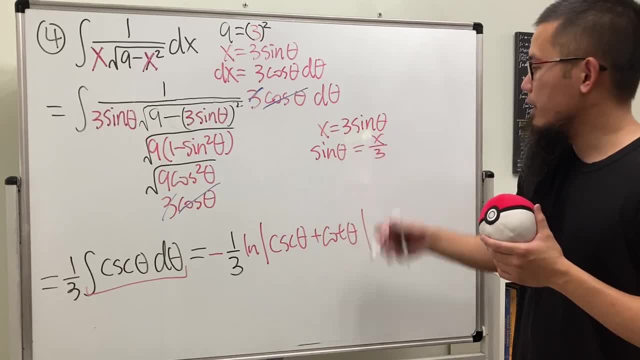 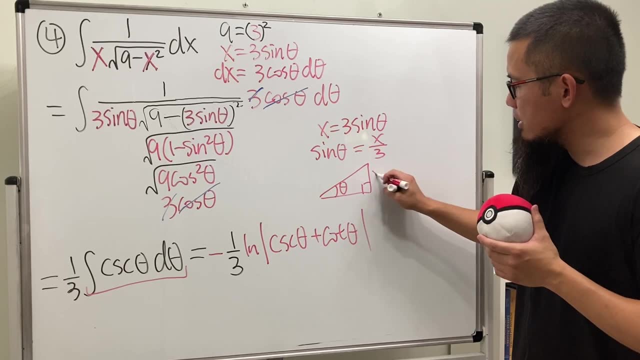 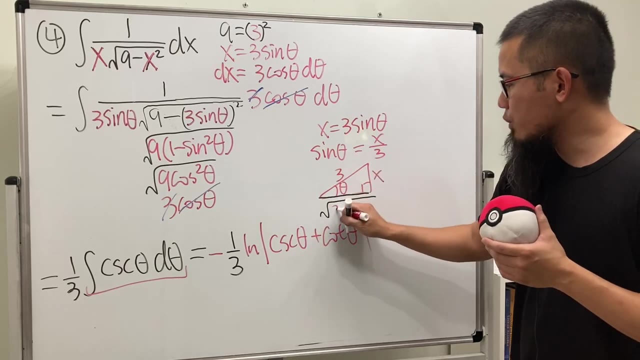 divide the 3 on both sides. so we're looking at this: draw a right triangle real quick, put the right angle here and the angle theta here, opposite, over hypotenuse, and then to figure out the adjacent, we open the square root and then we do this thing: square minus, this thing. 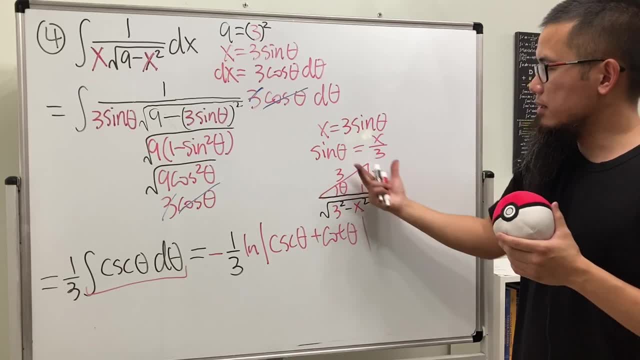 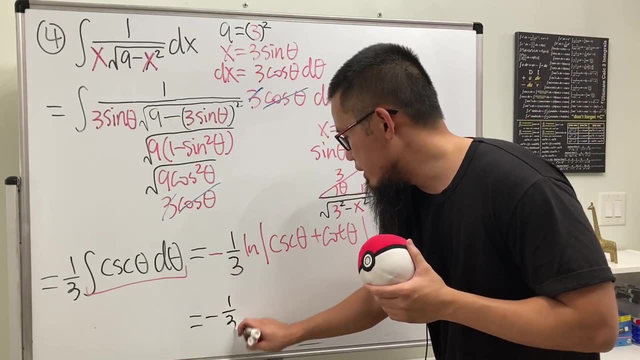 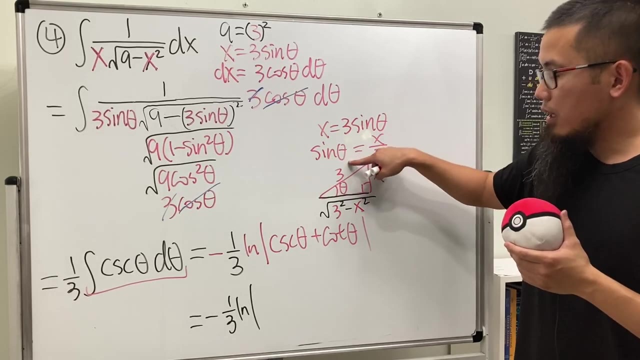 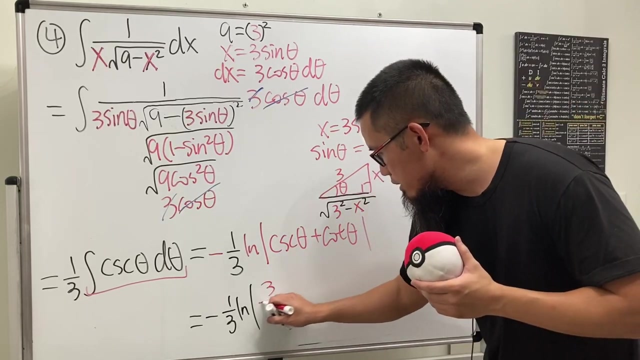 square. So this is the triangle that we have, and now we can just pretty much finish this. we have negative 1 over 3, ln, absolute value, cosecant theta. well, cosecant is just what hypotenuse over opposite. so we have 3 over x. it's quite strange, but that's just how it is. it is over. 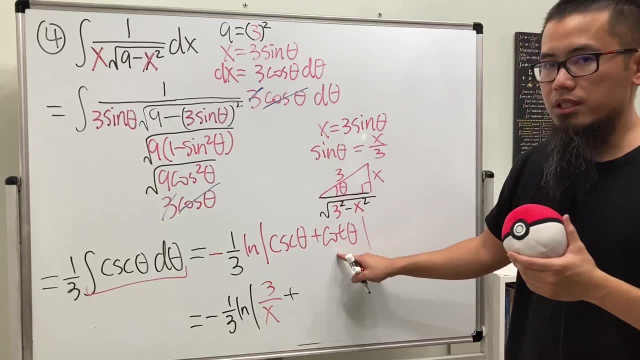 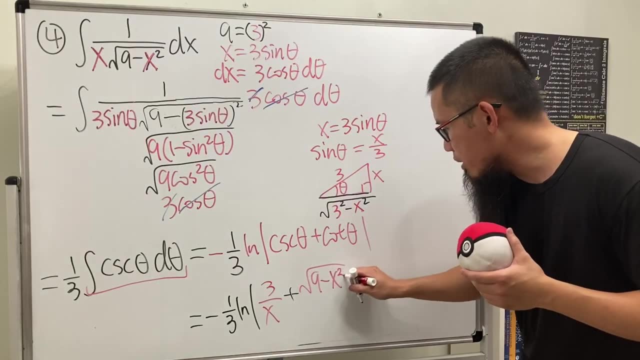 that. Next we are going to add cotangent. So we are going to add cotangent, which is this: over that right And this right here is just square root of 9, minus x squared and then over x. 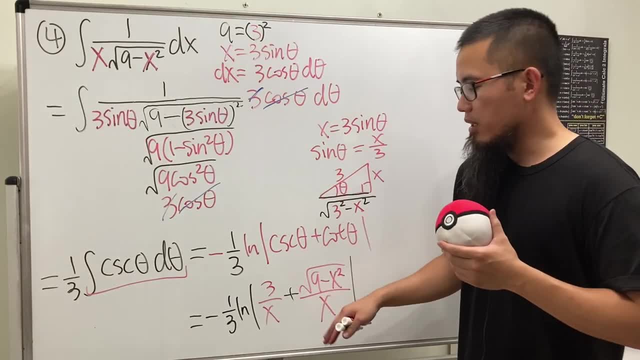 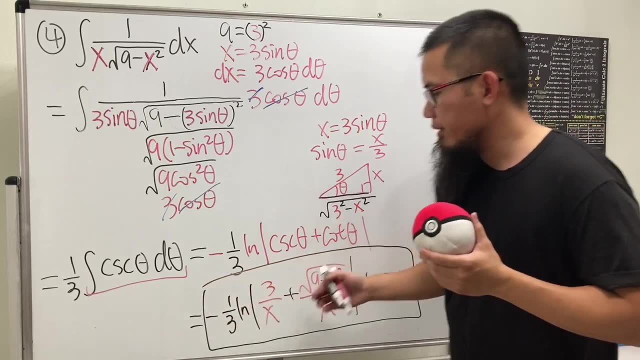 So that's pretty much it. of course you can also combine the x together and things like that, but I will just leave the answer like this: So put down the plus c, this right here is it Again. you might see people just have the negative right here instead of on the outside. 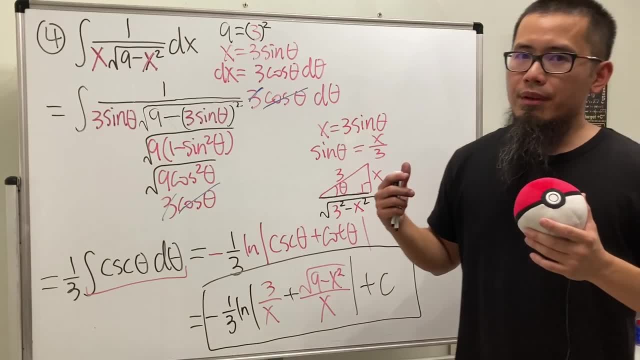 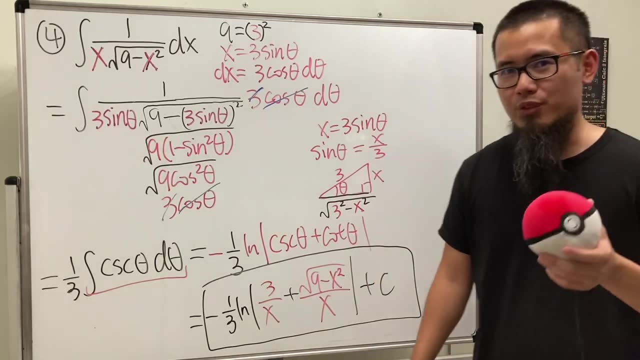 again same thing, alright, So hopefully this video helps. if you guys need more help, you guys know what to do. check out my other videos and also subscribe to the channel for future videos. and, as always, that's it.